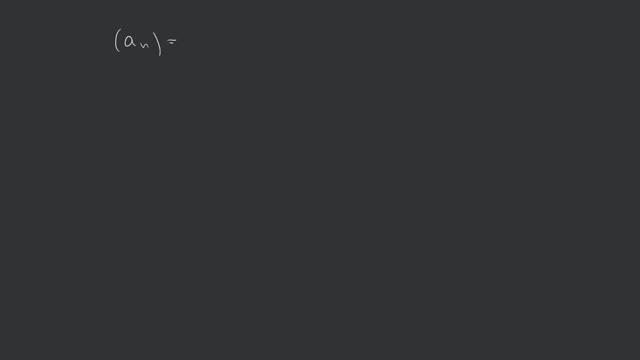 For instance, let's start with a: n equals n over n plus one. In fact, this is a very easy sequence and we can easily write down the first members, which is one half, two, third, three over four, four over five, five over six, and so on. 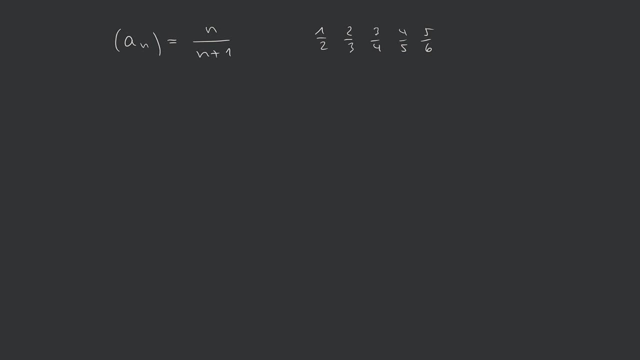 So you see, the denominator is always one higher than the numerator. It is very obvious that this sequence tends to one, But we want to find this result in a mathematically exact way. So we keep that as a guiding idea and do some manipulations to that n over n plus one expression. 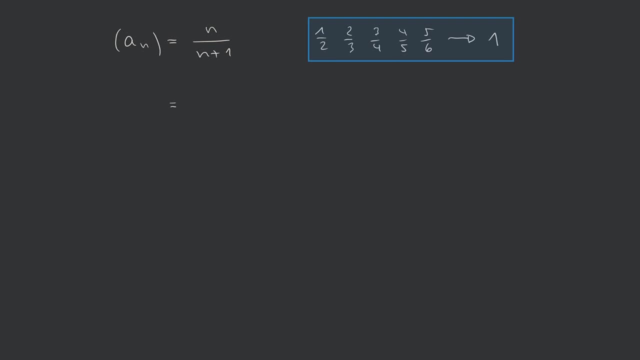 Now one first very important trick is that whenever a sequence is given by a fraction, that both for the numerator and the denominator, n should only occur in the denominator of the respective summons which occur in the numerator and the denominator. So let me show what I mean. 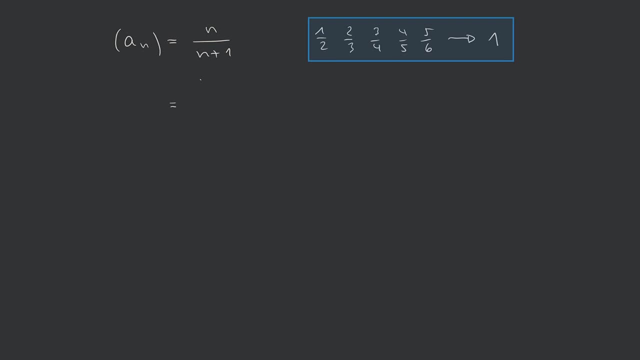 We reduce this fraction by n, So we get n over n, to do it very detailed, And again n over n plus one over n. So I reduce the fraction by n And of course now we can simplify, which is one over one plus one over n. 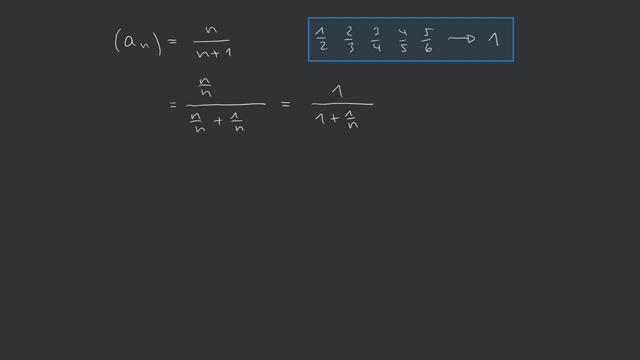 So now I have that situation, which I wanted, because n is only occurring in the denominator of the respective summons, Which is here In this denominator. Why do I want to achieve this situation? Well, this sequence, taken on its own, is a so-called zero sequence. 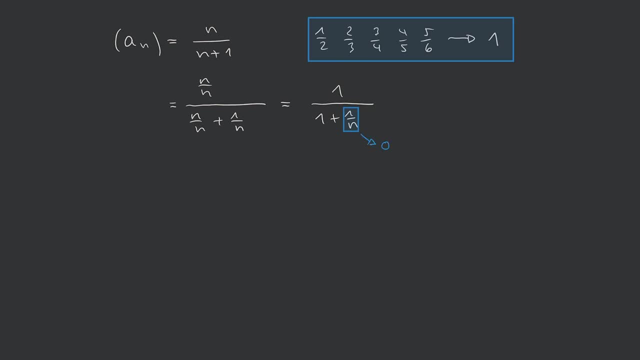 It has the limit zero. So if n goes to infinity, one over n tends to zero. So that is a well-known fact which we can use here in our argumentation. Now we apply the rules for limits, So that equation sign is due to the rules for limits. 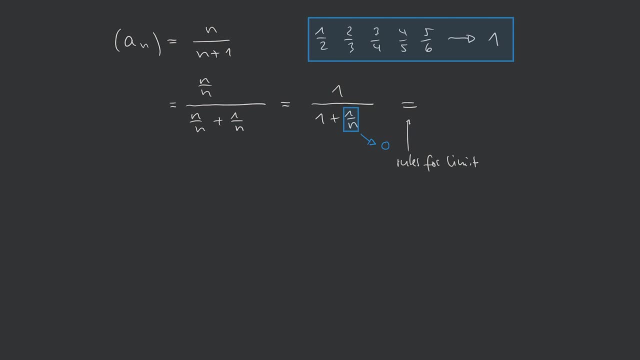 Because now we can split up Both the summation in the denominator and the big fraction, That means the division, And look at the limits separately. But the other sequences are very simple. This one can be considered to be the constant one sequence which of course goes to one. 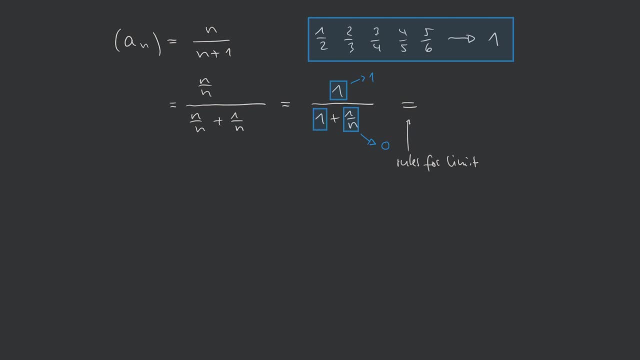 It's only one, one, one one, okay, And also this one has the limit one. So now the rules for limits allows us to split this up to one over one plus zero. So these blue numbers Are the respective limits of these three sequences. 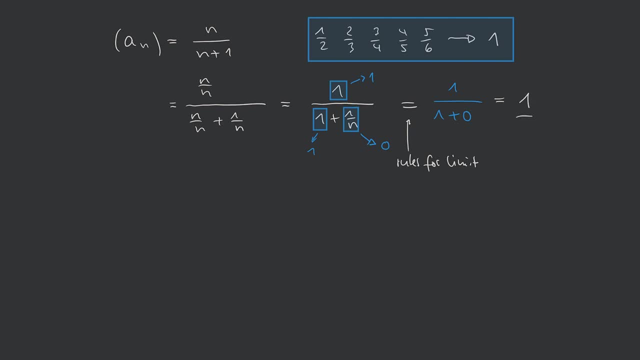 And finally, as the result, we get one over one, which is one. So the limit of that original sequence is one, and that coincides with what we already expected. As a second example, we look at the sequence a: n equals five and n to the third power plus. 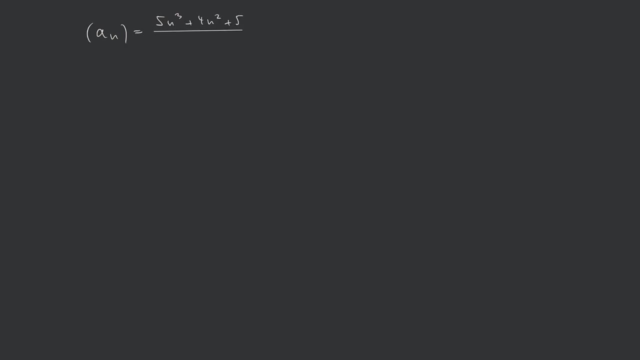 four And n to the second power plus five divided by two And n to the third power equals four power plus 8n. Again, the first thing we do here is to put n into the denominator of all these summands. We do this by identifying the summands with the highest power of n. These are those two. 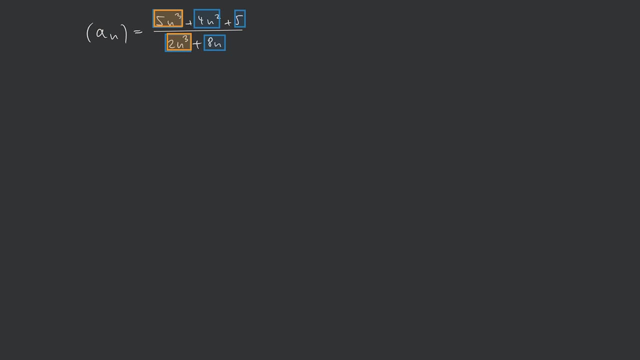 Here n occurs in the third power. Next we reduce the fraction by this highest power of n, in this case n to the third power. So we get the following fraction: 5 plus 4.. Now n to the. 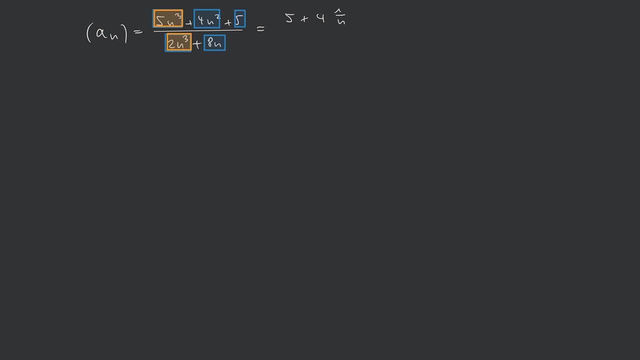 second power divided by n to the third power, is 1 over n, So 4 times 1 over n, plus 5 times 1 over n to the third power, divided by 2 plus 8 times 1 over n to the second power. So now we are ready. 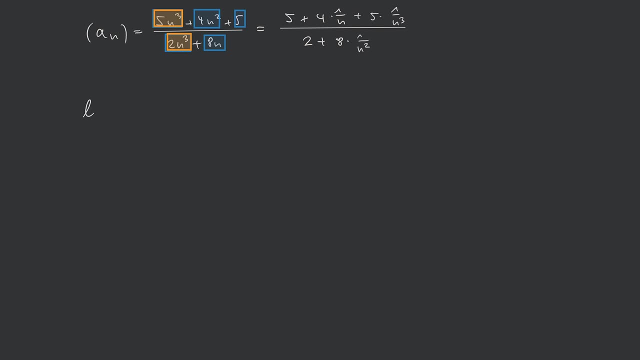 to apply the rules for limits. So I start. I start with lim for limit n to infinity of an equals. well, now we replace an by the fraction we have just calculated, which is 5 plus 4 times 1 over n plus 5 times 1 over n. to the third power: 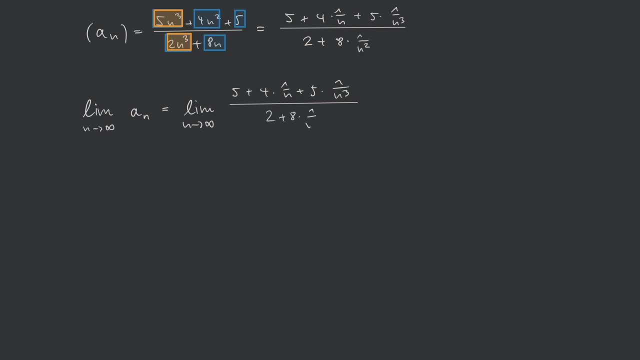 divided by 2 plus 8 times 1 over n to the second power. Now, using the rules for limits, we may distribute the lim n to infinity to the different summands in the numerator and the denominator of the fraction. So we get lim. Now I just leave away the n to infinity. okay, because that is taken for granted. 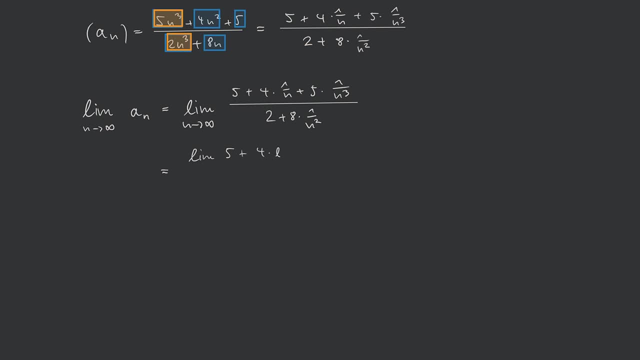 So I have lim 5 plus 4 times lim 1 over n plus 5 times lim 1 over n to the third power, divided by lim 2 plus 8 times lim 1 over n to the second power. Now, why did we do that? Because we know something about the limits of the sequences where n is still. 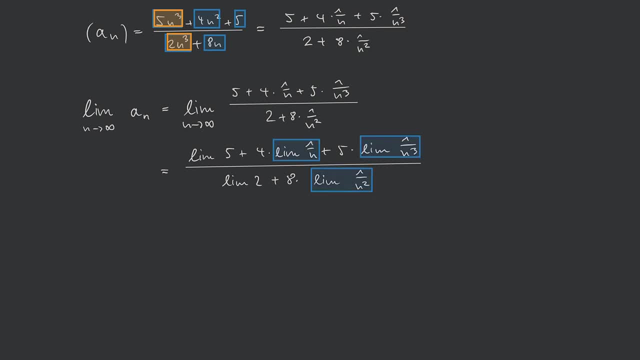 involved. These are these three. So what do we know about these sequences? Well, because n is in the denominator and not in the numerator anymore, all these three sequences are zero sequences. That means their limit is zero. The remaining two limits- lim 5 and lim 2, are limits of constant. 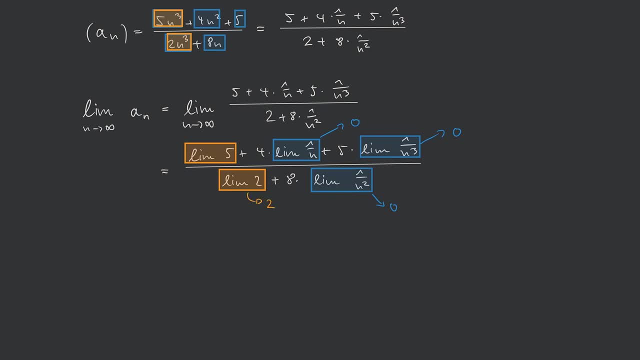 sequences. So the limits are very easy: That is 2 and that is 5.. So, using all these simplifications, we can write 5.. Plus well, the remaining summands in the numerator are both zero, So only 5 remains divided by 2.. 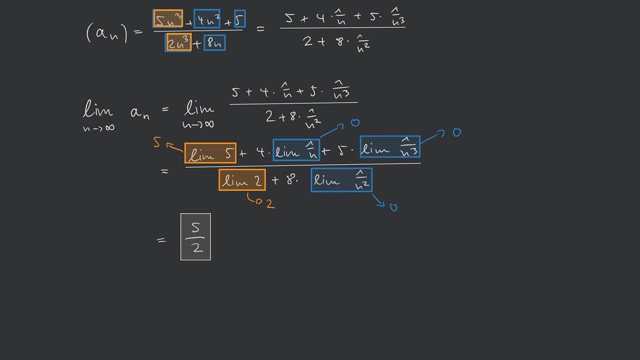 That's it. That is the limit of our sequence. There we go. So let us note that general rule. If we have a n equals 1 over n to the power of k, with k greater than zero, then we have that a n is a zero sequence. That means the lim n to infinity of a n. 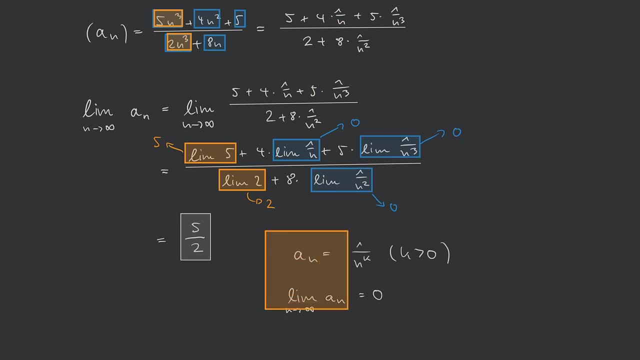 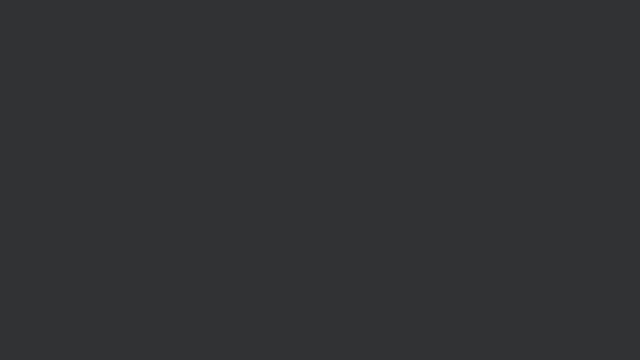 equals zero. That is a general rule which we used here in this example and in the example before. The next example we look at is the following sequence: a n equals square root of n plus 1 minus square root of n. This sequence can be thought of as the difference of two sequences. 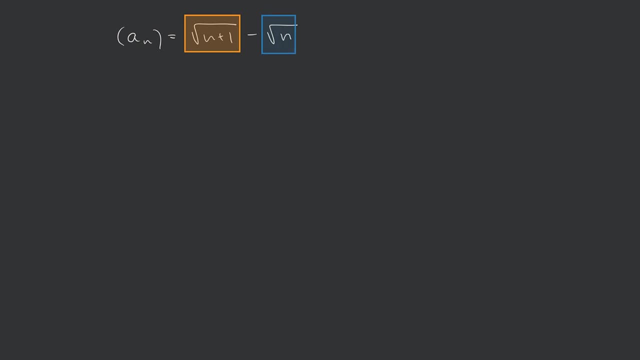 This is the first one and this is the second one. Let us call the first one b? n and the second one c n. Looking at the graphical representation of b? n- the orange points- and c n- the blue points- we see the typical shapes of square root functions, which is not surprising because we have the square 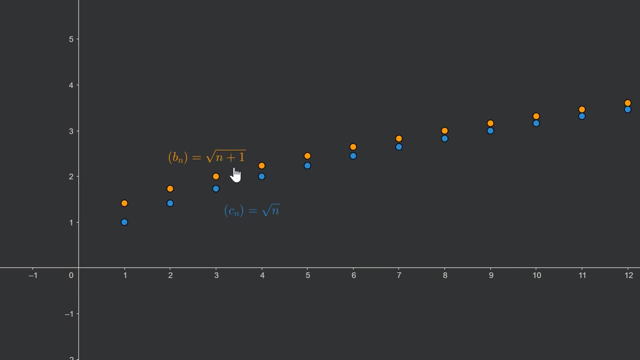 roots here. So the sequence we are interested in is the difference between b? n and c? n, and that is represented by the differences of these two points respectively. So the question is, is this a zero sequence? Because you can see, they approach each other more and more. 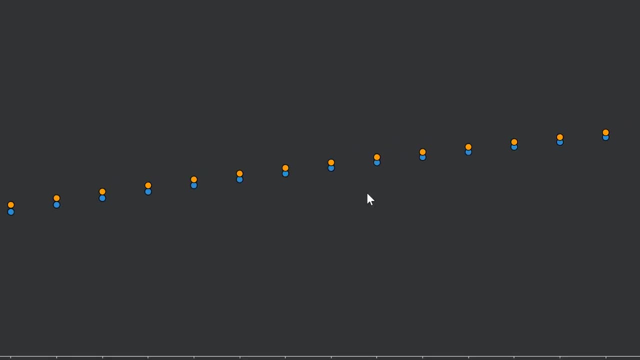 But that is only a graphical expectation. To know it for a sure, we have to prove it with a rigid mathematical approach. So let's do that Now. here we use a little trick. We multiply the formula of the sequence with this expression: Square root of n plus 1, and now plus square root of 1.. So we multiply. 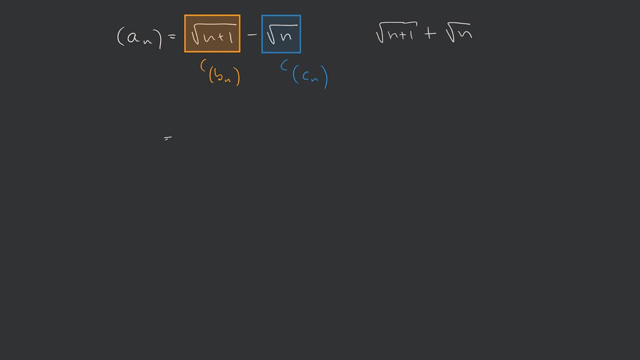 the expression by this expression and of course we have to redo that by again dividing it by this expression. Now let's see why we do that. So that is our original sequence, and we put that into brackets and multiply it with this new expression, which differs only by the sign here, And then we 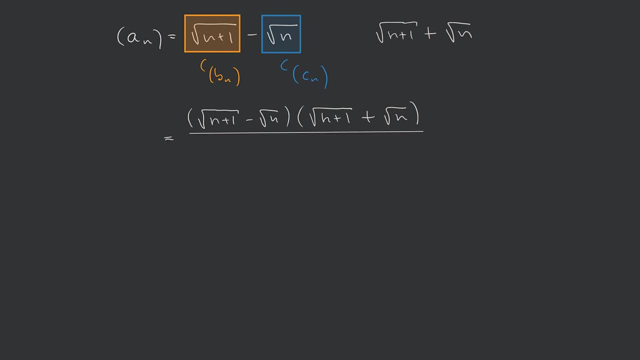 divide it by that expression again. So we write it here: n plus 1 plus square root of n. Now what should that be good for? The thing is that we can do something with this part. We can apply the third binomial formula. Now, let's recall the third binomial formula. It's: 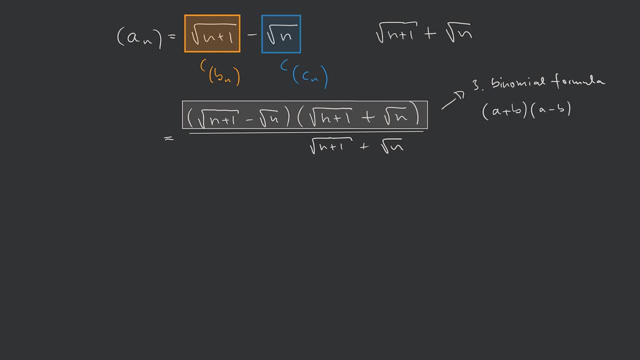 a plus b times a minus b equals a squared minus b squared. And if we apply that here, we find that we have n plus 1, which is the square of this expression, minus n, which is the square of this expression. And of course we have to divide this by the denominator. 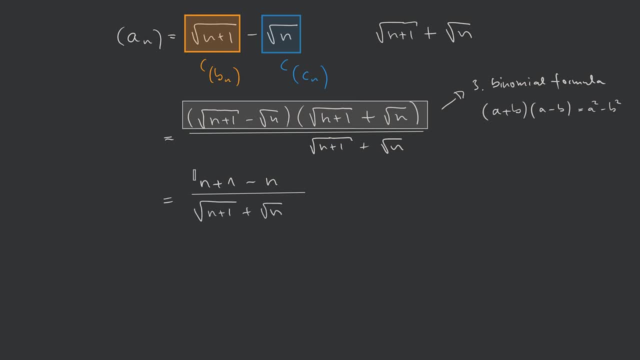 as above. But now the numerator gets very easy, because we have n plus 1 minus n, which is simply 0. So there's only the number 1 remaining, And you see how that simplifies. And we still have. 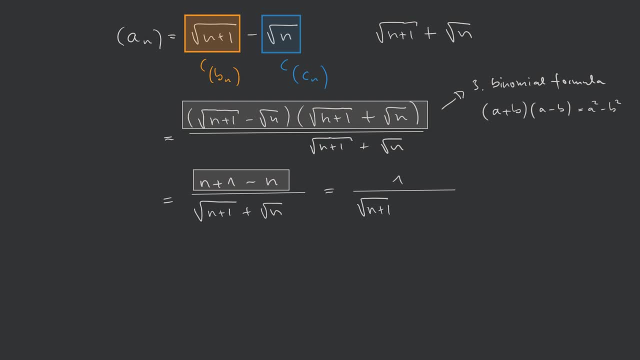 the denominator square root n plus 1 plus square root n. So now let's examine this expression in the yellow box more closely. First, it's easy to see that this expression is always greater than or equal to 0. So it never can get negative. Secondly, I want you to compare the expression: 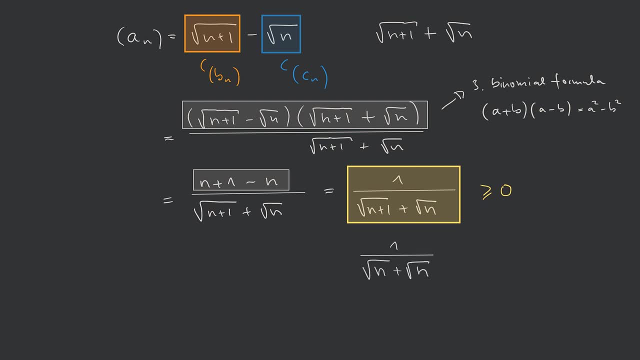 in the yellow box with this expression. What is the difference? Well, the difference is that we have replaced the square root of n plus 1 by the square root of n. Now, apparently, the expression which we used as a replacement is smaller than the expression which has been replaced, That is, smaller than the square root. 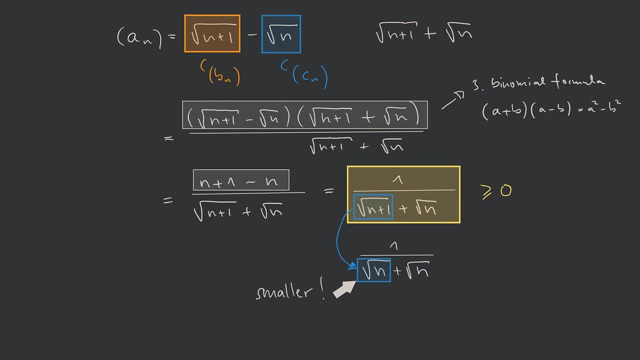 of n plus 1.. So altogether the denominator is smaller, which is why the expression in the orange box is greater than the expression in the yellow box. If we bring this all together, we have 1 over square root of n plus square root of n, which is the expression the orange box is greater than or. 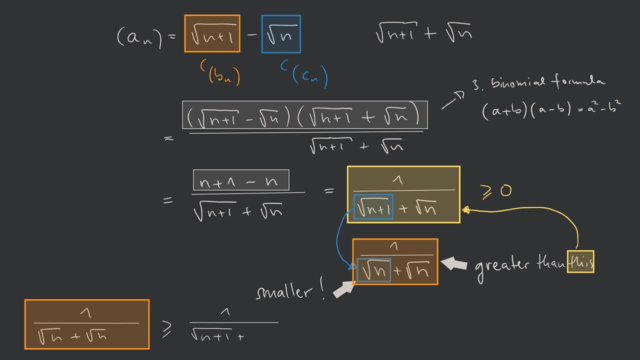 equal to 1 over square root of n plus 1, plus square root of n, which is the expression. the yellow box, which is greater than or equal to 0.. Now, if we look at the expression in the orange box, that can be simplified to: 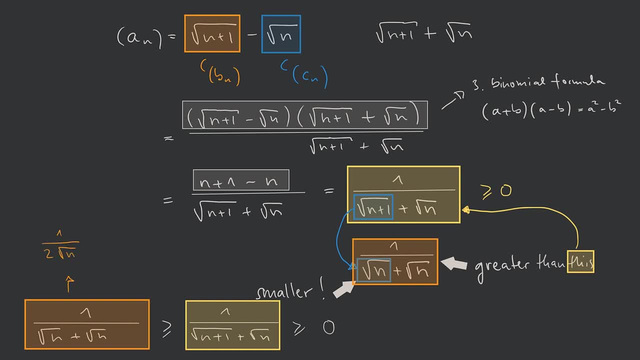 1 over of n. Now where does this sequence go? if n tends to infinity, That obviously is a zero sequence. So that goes to zero when n goes to infinity. So in mathematics that is called a squeezing trick, because we squeeze the expression in the yellow. 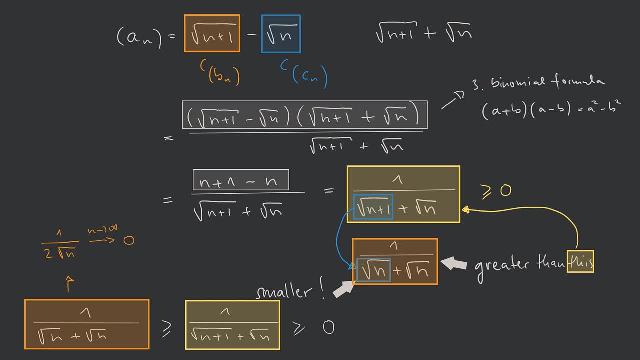 box between zero on the right hand side and a zero sequence on the left hand side. So, taking the limits we have, zero is greater than or equal lim n to infinity of our expression in the yellow box which we're interested in. So one over square root of n plus one plus square root of n, and again greater than. 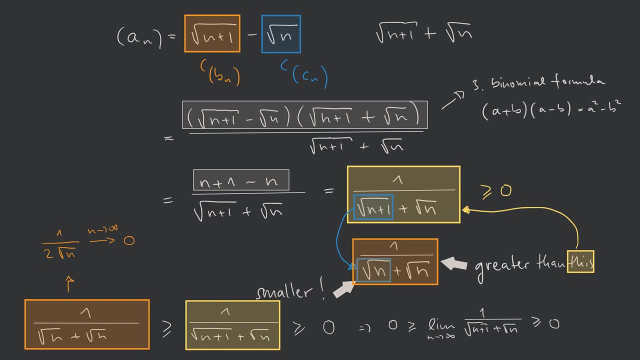 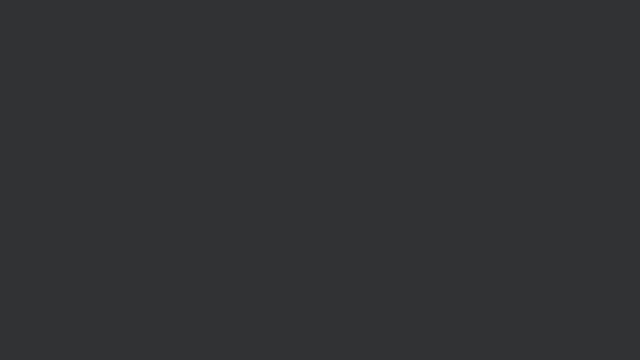 or equal zero. So see, it's being squeezed between two zeros, so that must also be zero. So the consequence is that the limit of a? n is 0. And that is in accordance with our expectation. Now let's do another example. A? n is equal to 5 for every x to the power of n. 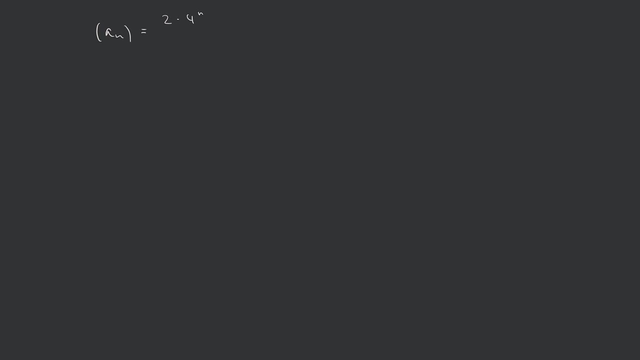 equals 2 times 4 to the power of n, plus 5 to the power of n plus 1, divided by 3 times 5 to the power of n, plus 7 times 2 to the power of n. So first note that they all are powers of n, except. 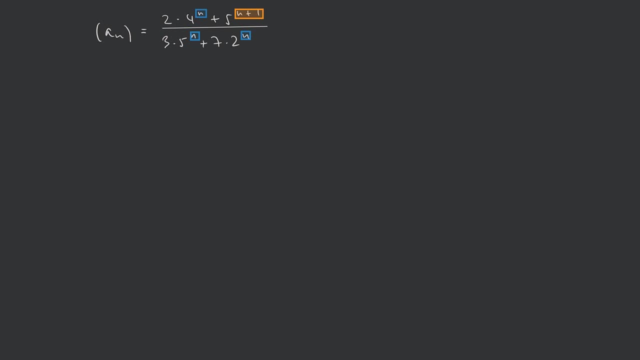 for 1n plus 1.. We can change this to n by splitting away one factor 5, what we do now. So we have 2 times 4 to the power of n, plus now 5 times 5 to the power of n. So that is the change and 3 times. 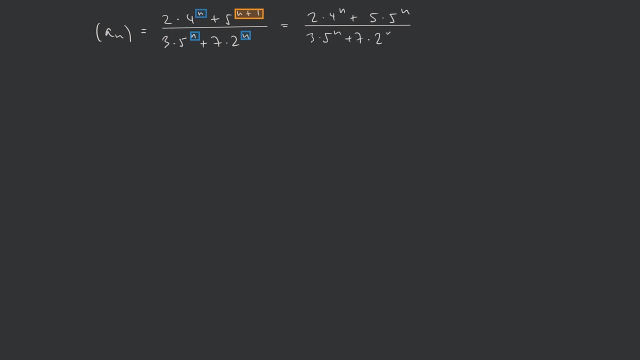 5 to the power of n plus 7 times 2 to the power of n. So now we only have expressions of some bases to the power of n. Now we choose those of these expressions with the highest bases. This is the basis 5 and we have two of them. The next step: we reduce by this expression. That means we reduce. 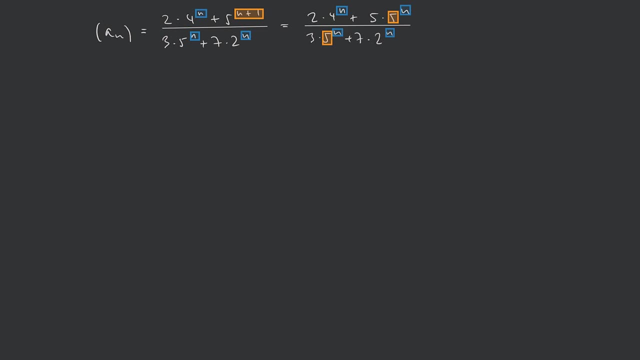 the fraction by 5 to the power of n. So we have 2 to the power of n. Now we choose those of these to the power of n, So we get 2 times 4 over 5 to the power of n plus 5, well, in this case 5 to the. 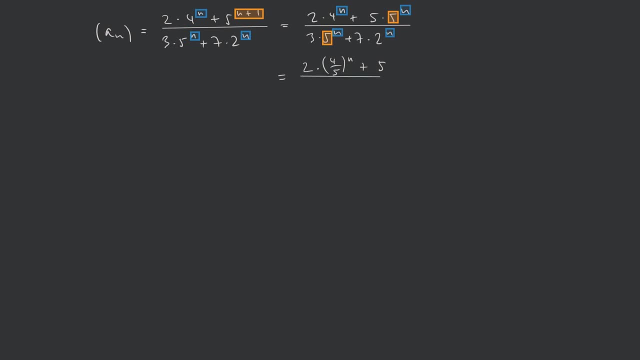 power of n cancels entirely out divided by 3, here 5 to the power of n also cancels out plus 7 times 2 over 5 to the power of n. So two sequences remain where n is involved, which is this one. 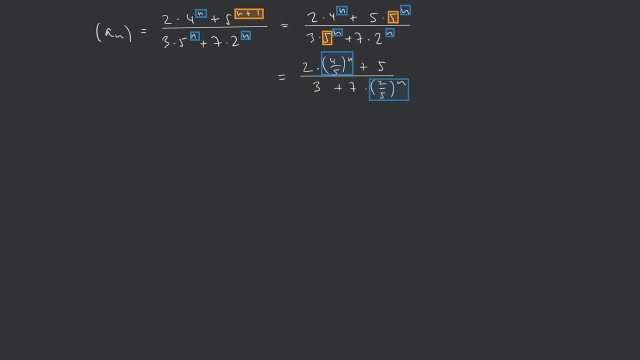 and this one. However, both of these sequences are of the form q to the power of n, with absolute value of q strictly smaller than 1.. And we already know that the limit of those sequences are always 0. So there are 0 sequences. That means 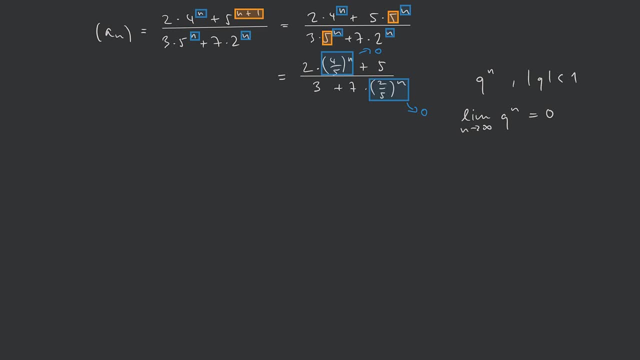 these two tend to 0,, such that in the limit. so I can't write an equation sign, but I can write something like n to infinity. So we get well, the first summand in the numerator just vanishes because we have the first summand in the numerator. So we have the first summand in the numerator. 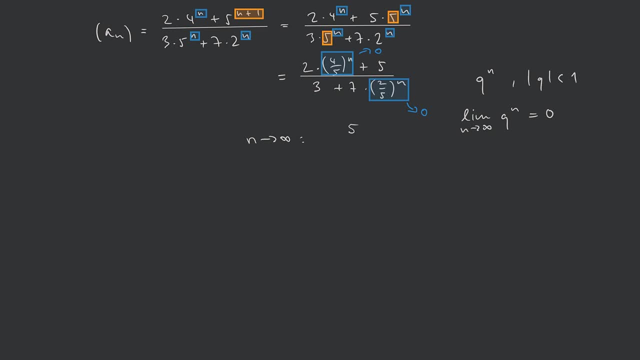 because it's a 0 sequence. So 5 remains and in the denominator the 3 is remaining and the other summand is vanishing because it goes to 0. So that is the limit of that sequence. Let's write that in. 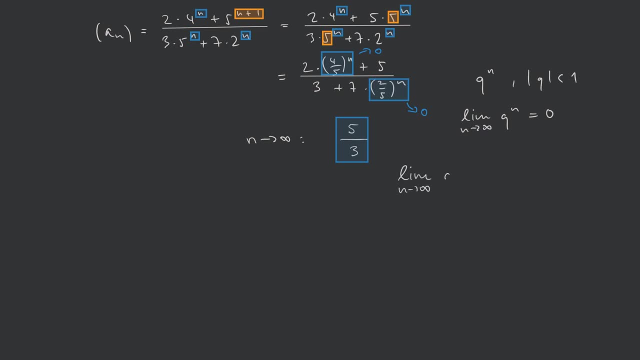 a nice way. So we have lim n to infinity of a n equals 5 over 3.. So let's look at the next example, which is a n equals 1 minus square root of n minus 1 over n, divided by 1 minus n minus 1 over n. So what can we do here? Well, the trick is: 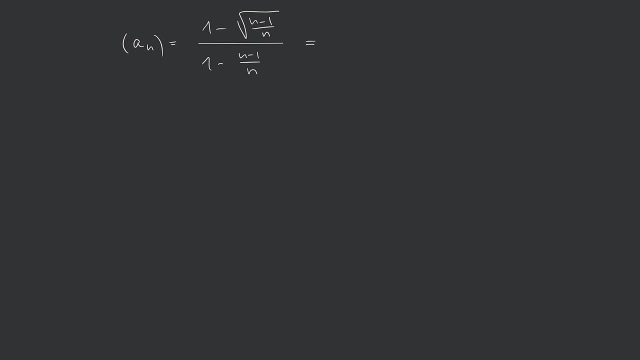 that we can apply the third binomial formula in order to reduce the fraction. Let me show you how that works. For reasons of simplicity, we first replace the expression n minus 1 over n by, let's call it b with. b equals n minus 1 over n. 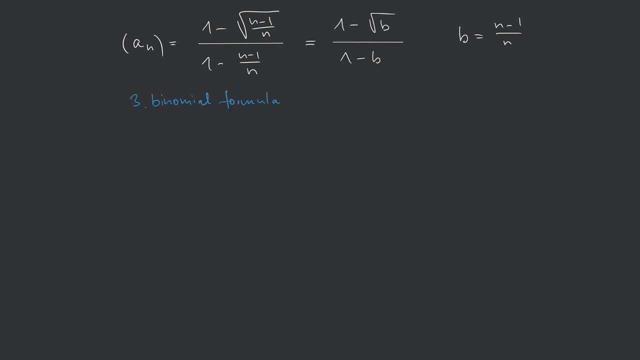 The third binomial formula allows us to split up 1 minus b into 1 minus square root of b times 1 plus square root of b. That is the third binomial formula. in this special case, We use this to split up the denominator in this fraction, So we can write: is equal to 1 minus. 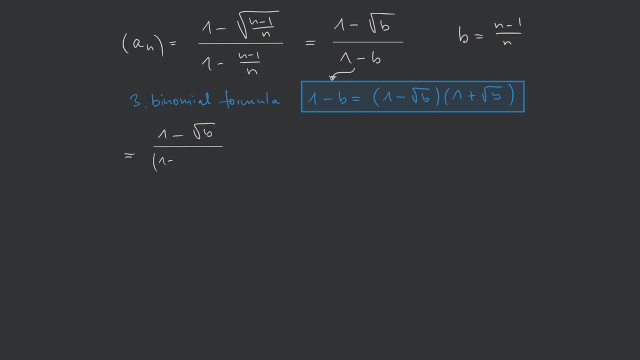 square root of b divided by 1 minus square root of b times 1 plus square root of b. In this fraction, the expression 1 minus square root of b occurs in the numerator and in the denominator, So we can reduce the fraction by this expression, which gives 1 over 1 plus square root of b. 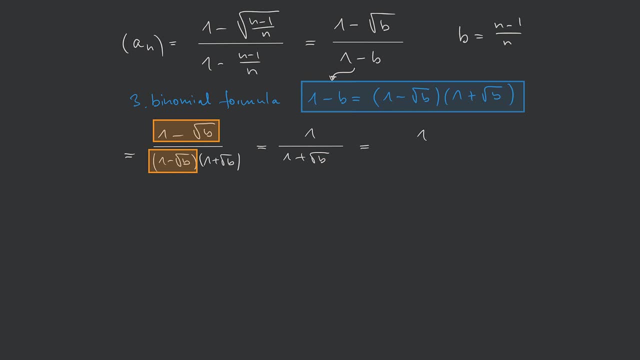 And if we re-substitute b, we get 1 over 1 plus square root of n minus 1 over n. Now we can start splitting up the limits. So let's write lim n to infinity of b to infinity of a. n equals lim one over lim one plus lim, square root of n minus one over n. 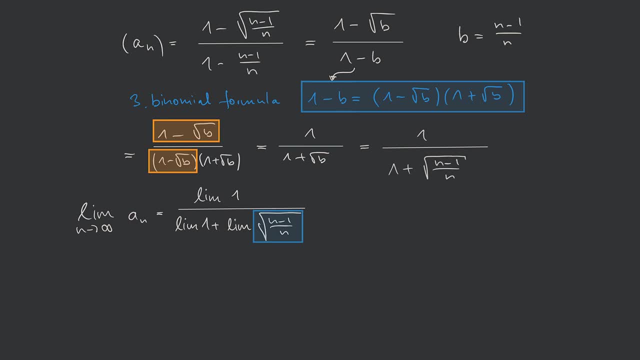 Now, the only interesting part here is this one, And we need to find out what the limit of that sequence is. So where does the expression under the square root go to? This expression is n minus one over n. Where does this go to? Well, we can split that fraction up into n over n minus one. 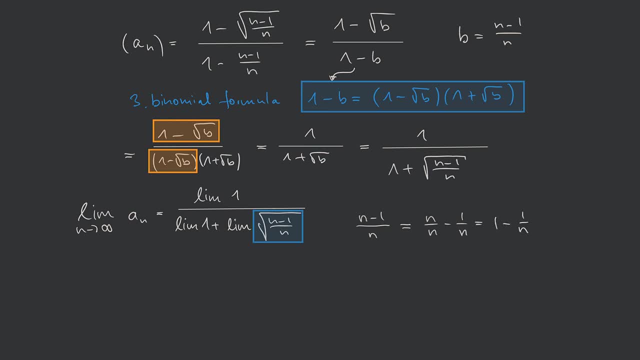 over n, which is one minus one over n. One over n, however, is a zero sequence, so this goes to zero. So what remains in the limit is if n goes to infinity is one. So if the limit of the sequence 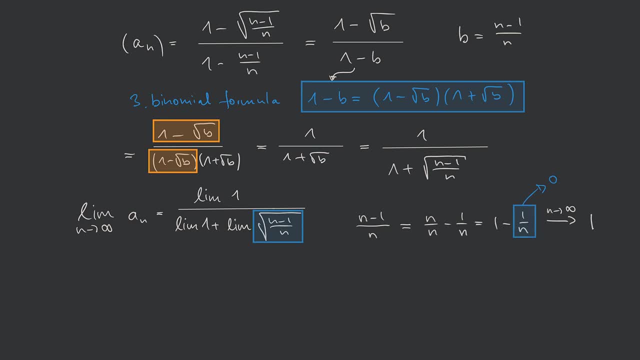 under the square root is one. the limit of the sequence itself is also one. So we have that this limit is one. Putting it all together gives one over one plus one, which is one over n, minus one over n, which is one over n minus one over n. 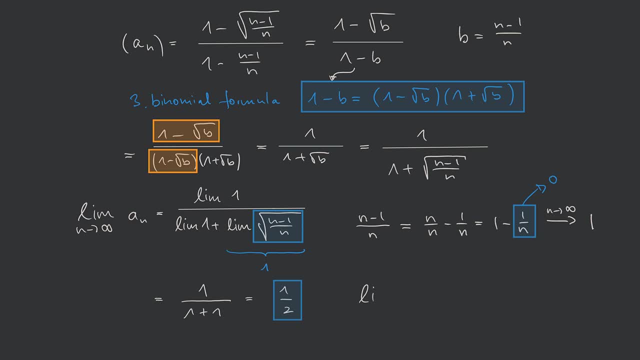 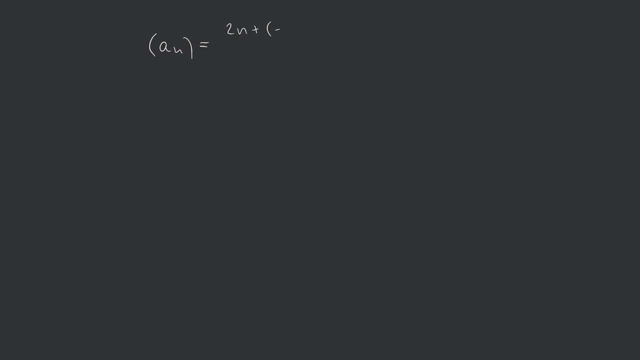 So the limit of a? n equals one half. Admittedly, the trick with a binomial formula is a bit hard to see, So that is a trick one has to keep in mind whenever you come across a similar sequence. Next we look at the sequence a? n equals two n plus minus one to the power of n. 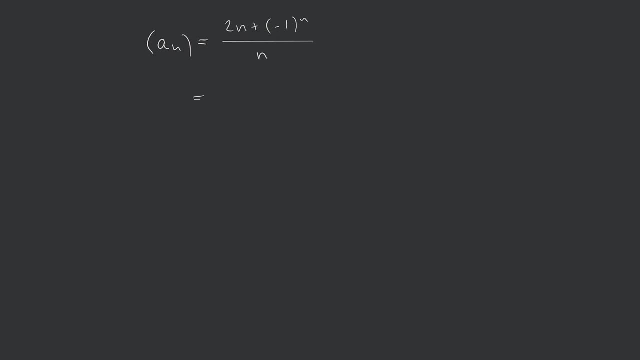 divided by n. This one is comparably simple because we can split up the fraction to well, two n over n, plus minus one to the power of n over n, And of course the first summand just reduces to two, which gives us two plus minus one to the power. 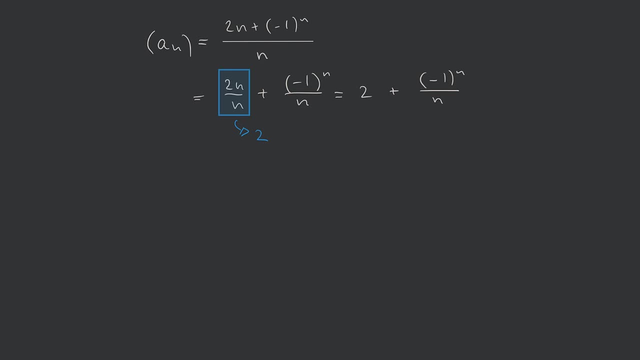 of n over n. Now, the only component in this formula which contains n is this one, And it's fruitful to understand how it behaves. Well, what does the numerator do? It is minus one to the power of n, So for n equals one. we have one over n, minus one to the power of n over n, So we have one over. 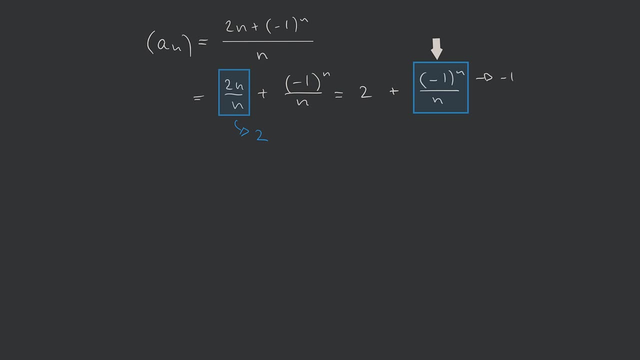 n minus one. we have minus one, For n equals two. we have minus one times minus one, which is one, For n equals three. we have minus one times minus one times minus one, which is minus one again. So you see that sequence oscillates between one and minus one forever, And of course, 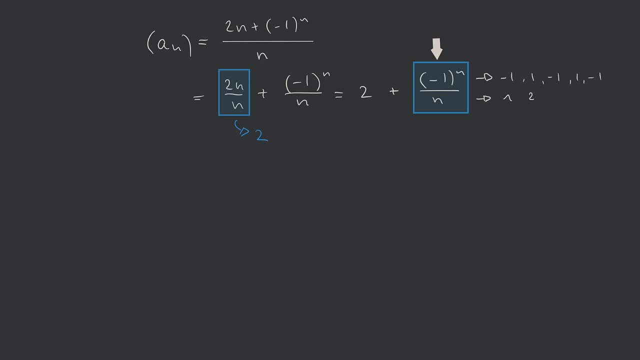 what happens in the denominator? that is easy, that is one, two, three, four and so on. So altogether we have a sequence which looks like minus one over one, one over two, minus one over three, one over four, minus one over five, and so on. So where does this go to? 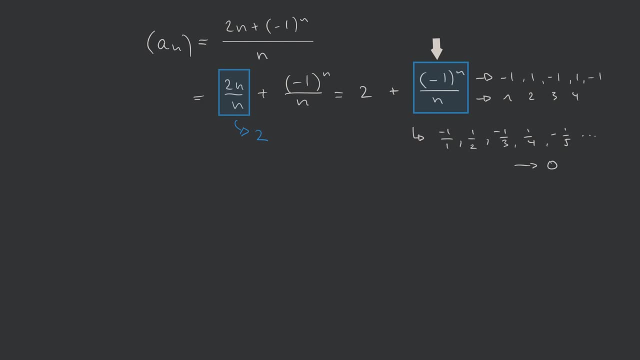 Well, obviously it goes to zero, So that is a zero sequence, just as if we didn't have the minus signs. Without the minus signs, the sequence looks like this, just roughly sketched And with the minus signs, well, the sequence looks like this, and then this jumps down here: 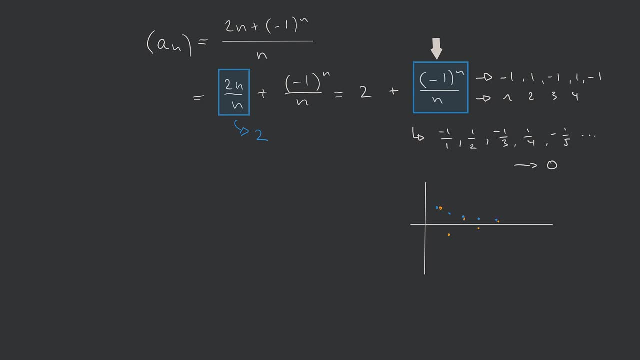 and then we go up here, and this one comes down here, and then we go up here. So you see, it moves around the zero line, but it's still a zero sequence. So that means that when n goes to infinity, this goes to zero, for n goes to infinity. 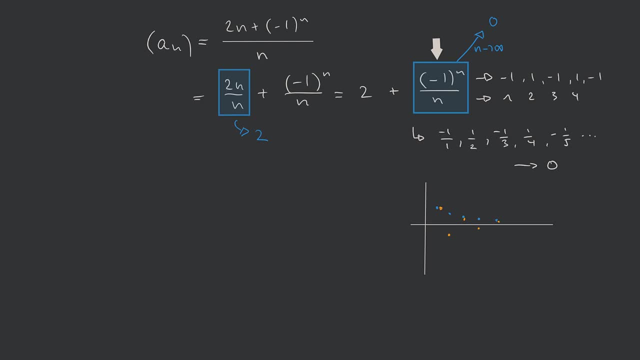 So altogether the limit of our sequence is two. So I can't write equals two, but I can write goes to two, for n goes to infinity. or the detailed way is lim n to infinity of a n equals two. And before you get bored, we jump to the next example, which is an equals two minus 3n over. 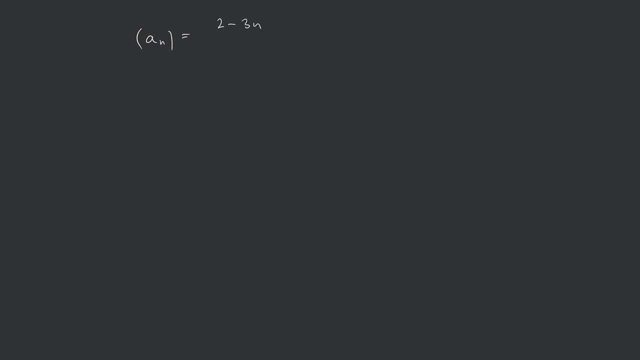 one plus four n, and we put that into brackets and square this expression. So that is our sequence. Now how can we treat that? Well, of course we can resolve the square by multiplying both the number and the value, here with itself, and the denominator with itself, and we will get more complicated. 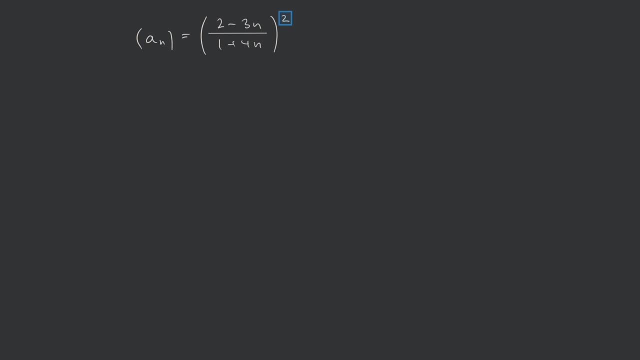 expressions in the numerator and the denominator. However, a better way is to first ignore the square and calculate the limit of this expression inside of the brackets, And as soon we have this, we apply one of our rules for limits and get the limit for the squared version. So let's see what happens with 2 minus 3n. 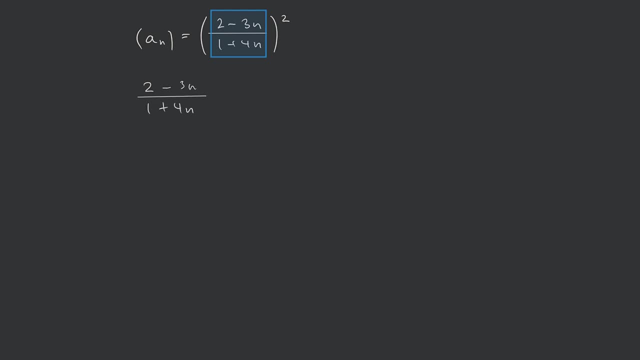 over 1 plus 4n. Again, we don't like n to be in the numerator of the respective summons. so we don't like n to be here. We rather want n to be in the denominator of the respective summons. so that is why we reduce this fraction by n, which is: 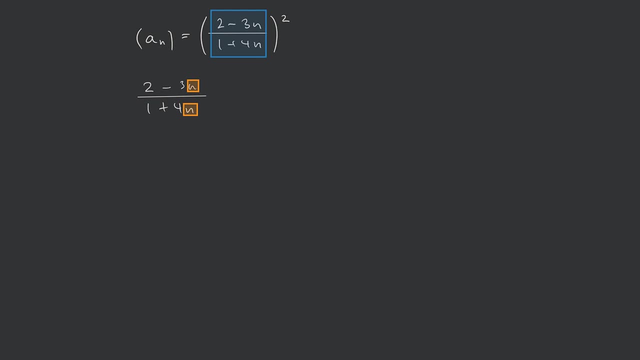 actually n to the first power, and that is the highest power of n. That is the rule of our previous examples: we just reduce the fraction by the highest power, highest power of n, which is n in this case. And what do we get? Well, we get 2. 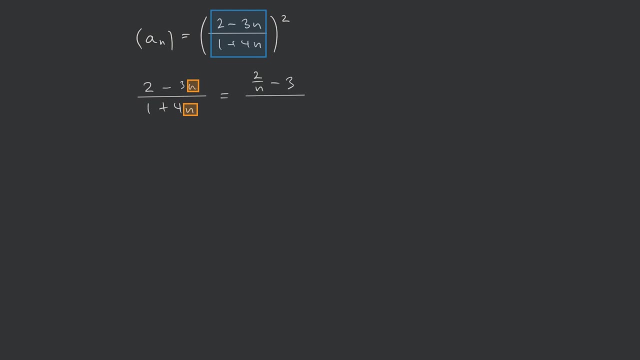 over n minus 3, divided by 1 over n plus 4.. And, following our old scheme, we know that this and this are zero sequences, so this goes to 0 and this goes to 0, and, in the limit so tending to, when n goes to infinity, this tends to minus 3.. 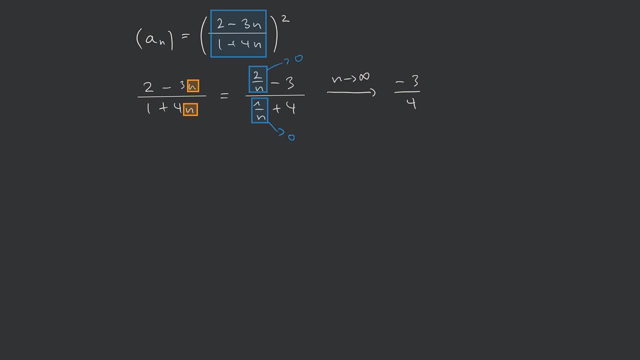 So we have 2 minus 3 over 4, which is the limit for the expression within the brackets. Now, from our rules for limits, we have lim n to infinity. an equals. well now, lim n to infinity of the expression above with the brackets. so 2 minus 3n. 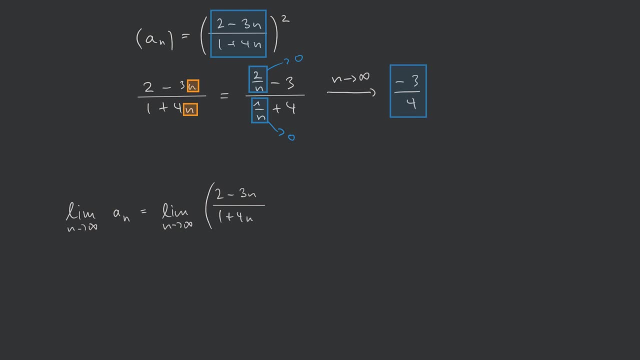 over 1 plus 4n squared. And now, because this is a square of two expressions and it's actually a multiplication of two sequences, we can split up the lim on these two sequences, So lim of the first one, which is actually this expression, without the square times. 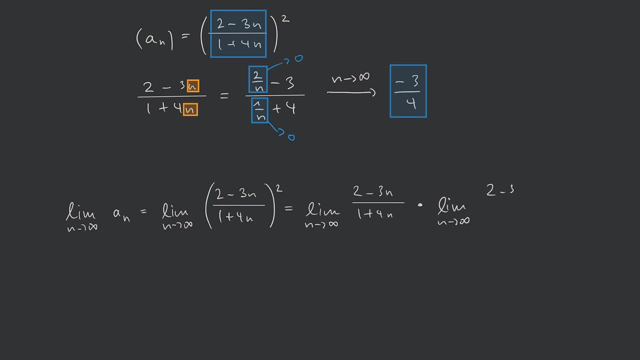 the same expression again. So let's repeat that We could use the square symbol, but let's just do this for reason of clarity. But this is already known to us, because those two are minus 3 over 4, respectively, So we 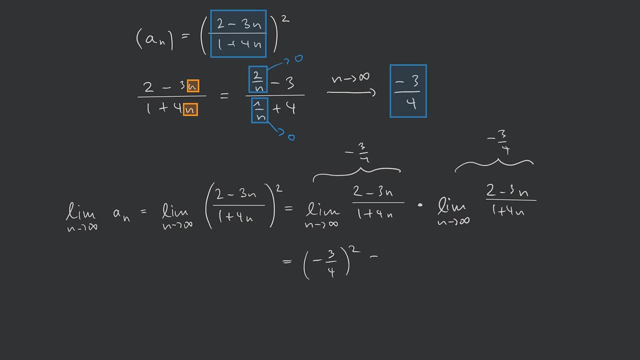 get minus 3 over 4, squared, which is 9 over 16.. And that is the limit of our sequence. Now, before we all get tired, we do the next example, which is an equals 1 plus 2 plus dot, dot, dot plus n divided by n plus 10 times square root of n squared minus n plus 1.. Well, 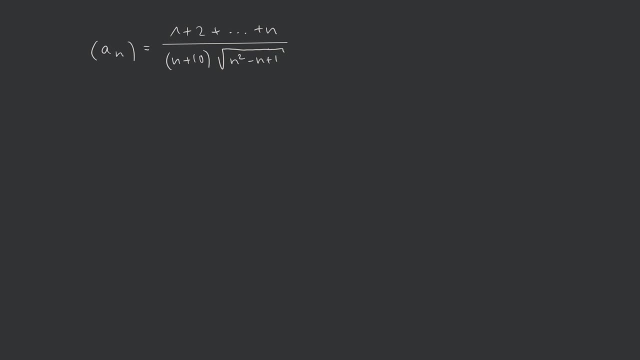 that's a mean one, Because there are some ingredients which we all have to tackle before we find the limit. So the first thing we should discover is that the so-called little goes is involved, which is the sum of the first n natural numbers. 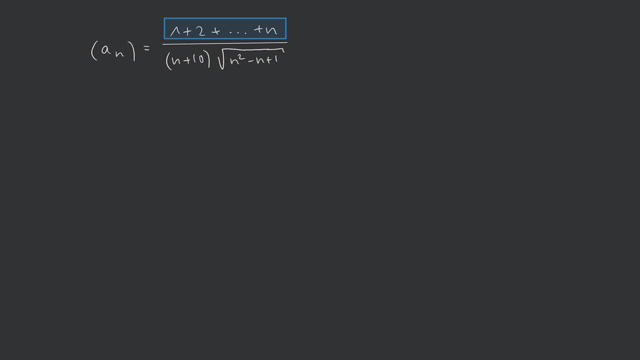 So if you're not sure what I mean, just watch the video for the little goes we did earlier. So that sum equals the expression n plus 1 times n over 2.. That is what the little goes is all about. So we replace the numerator by that new blue expression and we get the following. We get: 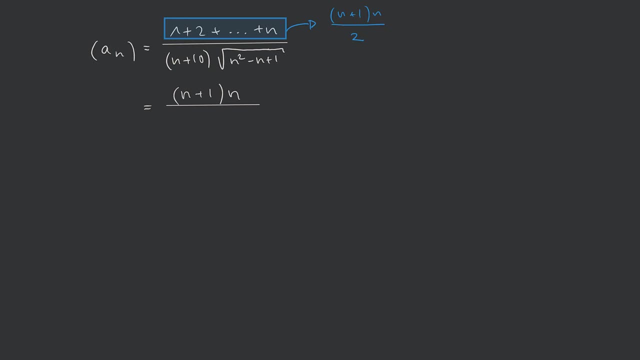 n plus 1 times n, divided by 2 times n plus 10 times the square root. In the next step we do all the multiplications both in the numerator and the denominator. That means we break up the brackets by expanding the multiplications. That means we have n squared. 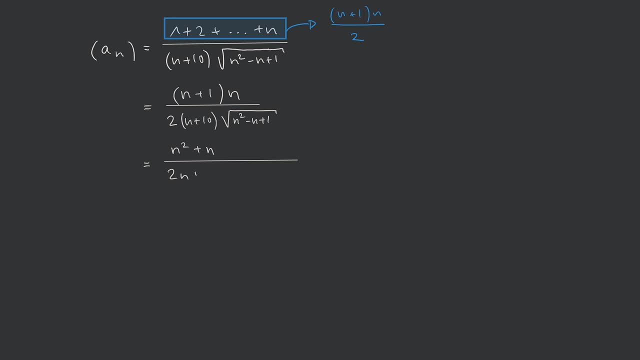 in the numerator and we have 2n times that long square root plus 20, and again the long square root. Now we follow the standard rule we know from our examples before, which is we figure out the highest exponent of n in these summands and reduce by this exponent, So that is n. 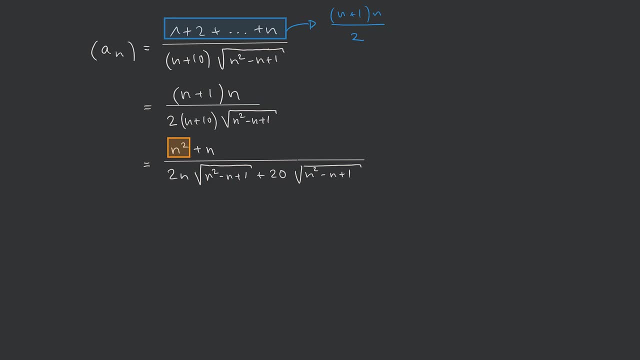 squared. So we reduce the fraction by n squared. That gives 1 plus 1 over n divided by. and now we have to be careful with the denominator. So there are two summands in the denominator and we have to divide each summand by n squared. 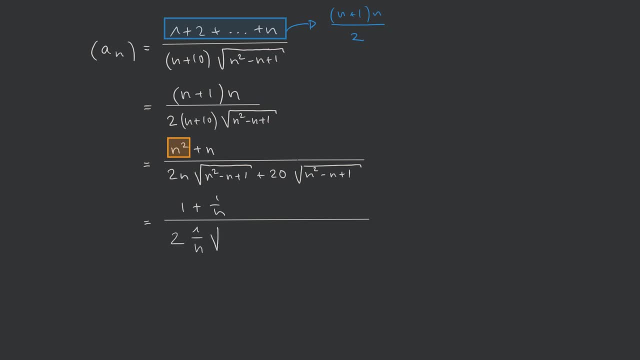 So the first will give 2 times 1 over n, then the long square root, plus 20 times 1 over n squared, then the long square root. Now what can I do with these two expressions? The idea is to take them under the square roots by first taking the square of them and 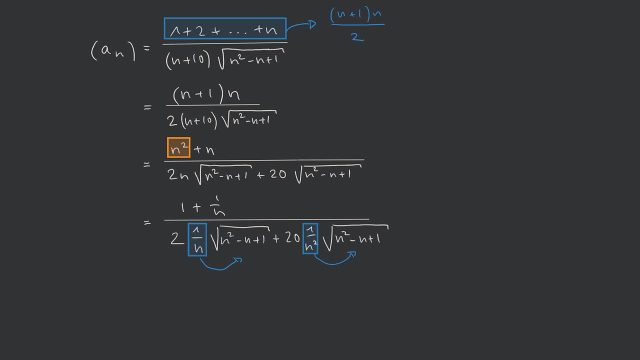 then taking them into the square root. So first we square both of these expressions- let me write it like this: we square them, and then we multiply them into the expression under the square root. This gives 1 plus 1 over n divided by 2 times. 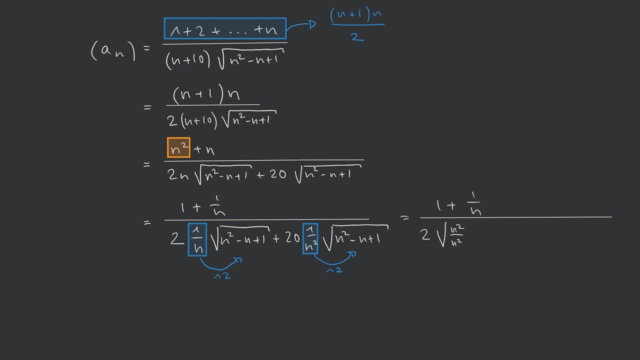 Now 1 over n is 1 over n squared. Now 1 over n is 1 over n squared. So we get n squared divided by n squared, minus n divided by n squared, plus 1 divided by n squared, That is the first square root. 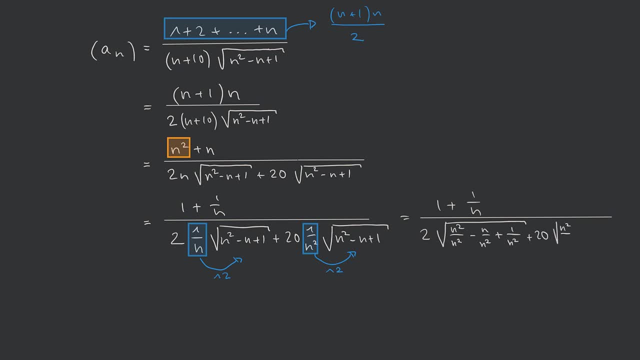 Then we have 20 and n squared. Now we divide by 1 over n squared times 1 over n squared is 1 over n to the 4th power. So that is the quotient we have here: n over n to the 4th power, plus 1 over n to the 4th. 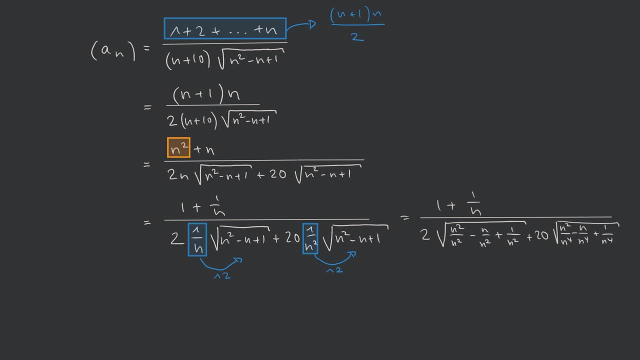 power. that's it Now. in the next step, we of course can simplify many of these terms in here. So we get 1 plus 1 over n divided by 2.. Now the first summand reduces to 1, the second summand reduces to 1 over n and the third stays as it is: 1 over n squared. That's the. 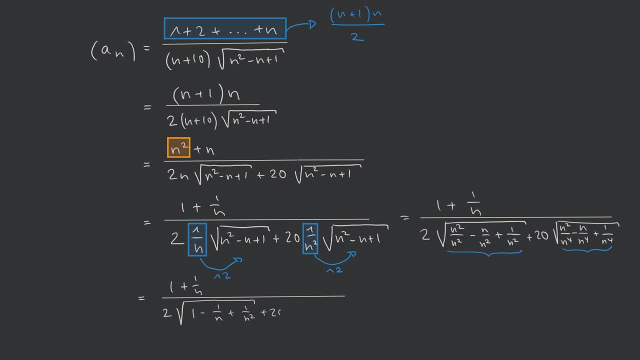 first square root and the second one is plus 20.. Now the first reduces to 1 over n squared, the second reduces to 1 over n to the third power, and the third one stays as it is: 1 over n to the fourth power. Now it's time to check what happens if n goes to infinity. 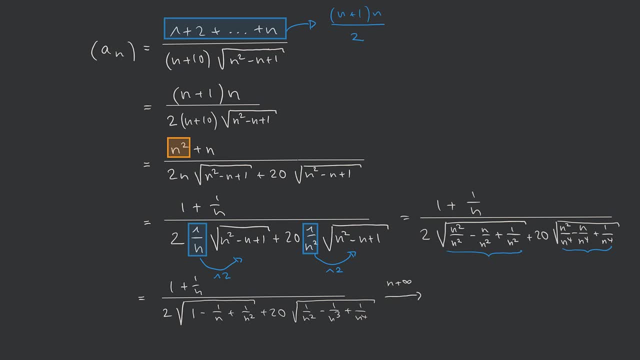 What happens? We have a lot of zero sequences here. First one is this one and there's another one, here's another one, here's another one, here's another one and here's another one. They all go to zero. So when n goes to infinity, 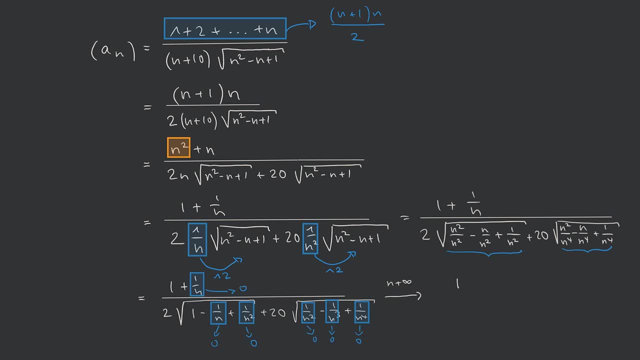 So let's collect what remains In the numerator. only the number 1 remains In the denominator. we have 2 times square root of, well, square root of 1, plus 20 times square root of. ooh, everything goes to zero. So square root of zero, So that part is zero, That part of course. 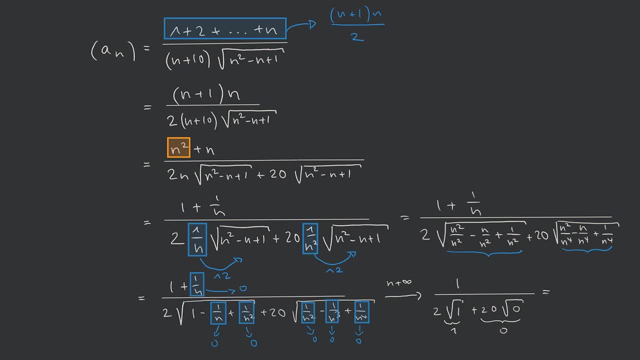 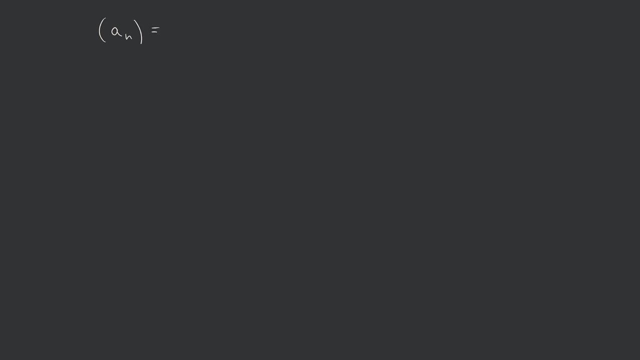 is 1.. So what remains? 1 over 2.. That's it. The limit of that complicated sequence is 1 half. Okay, so you're still with me. I have another one, which is: a: n equals n factorial over. 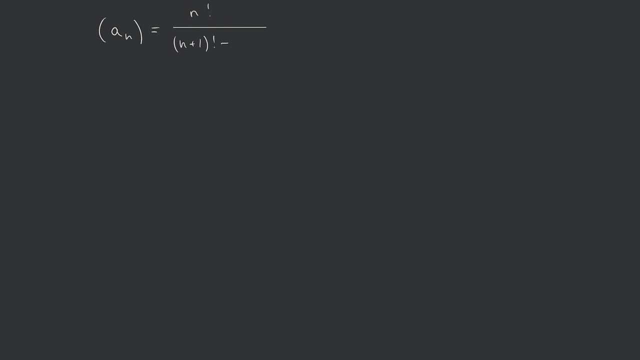 n plus 1 factorial minus n factorial. Ooh, that one looks very bad. So many factorials, But actually that is not bad at all. We just need to understand what factorial is. Just if you don't recall, 5 factorial is 5 times 4 times 3 times 2 times 1.. So actually something very easy. 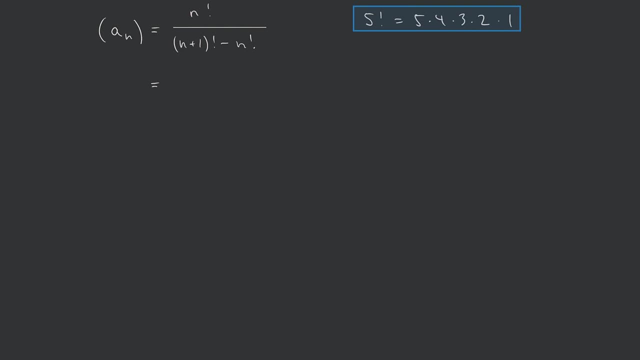 Now the trick here is that we need to understand that we can do something with this n plus 1 factorial, Because the only difference between n factorial and n plus 1 factorial, well, it's just like the only difference between 6 factorial and 5.. 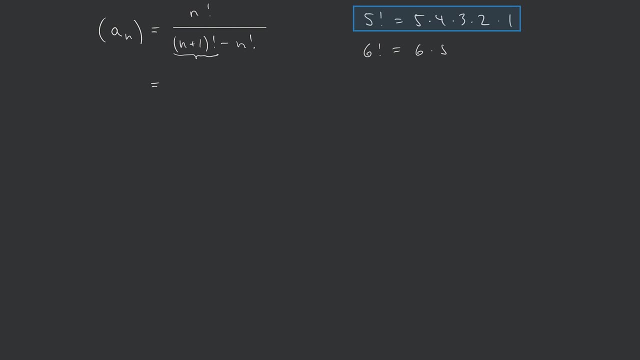 What is the only difference? Well, it's another 6.. The rest is the same. So this is 5 factorial and the only difference is this: 6 times 5 factorial. So, following this idea, we just can write nfaculty over n plus 1 times nfaculty. That: 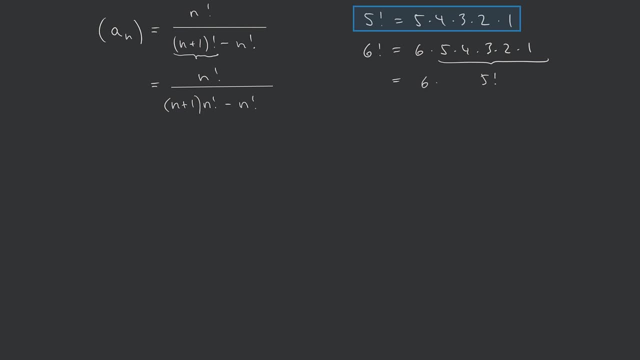 is the trick. And now minus nfaculty. And now it's obvious that we can reduce this fraction very efficiently, because we can reduce the fraction by nfaculty, which is 1 in the numerator, and n plus 1, minus 1 in the denominator, which results in 1 over n, And that's all, And we know already. 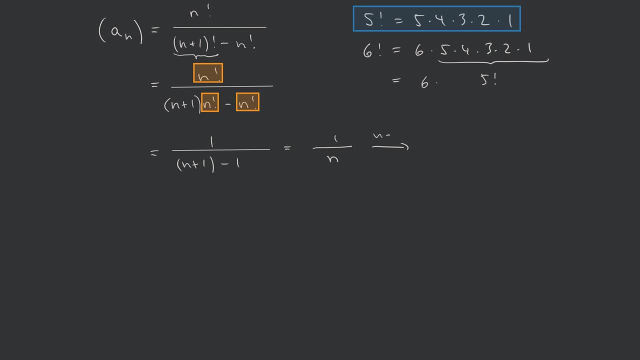 that 1 over n is something very simple. It's a zero sequence. So if n tends to infinity, we have zero as the limit. So that was a quick one. So as you are probably asleep by now, let's do a little harder one, which is a n, And now 1 plus 2 plus 3.. Yes, that sounds like the. 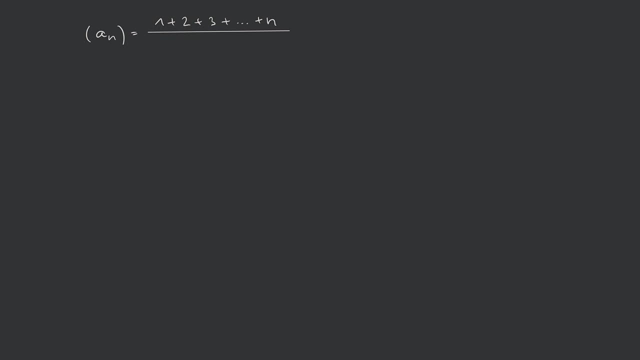 little gauss, again Plus n, divided by n plus 2, minus n over 2.. Now, as I already said, we have the situation as in one of our previous examples, because this sum here can be calculated using the little gauss. That means using this formula: n times n plus 1 over 2.. That is well. 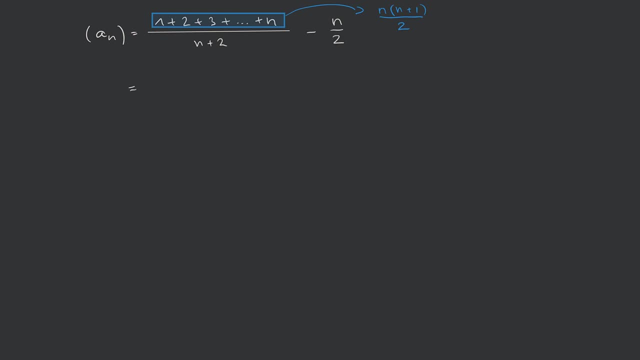 known by now, And we use this to get the following: I simply replace the sum in the blue box by this formula And we get the following: I simply replace the sum in the blue box by this formula And we get n times n plus 1 over 2 n plus 2.. So mind the 2, which is now in the denominator. 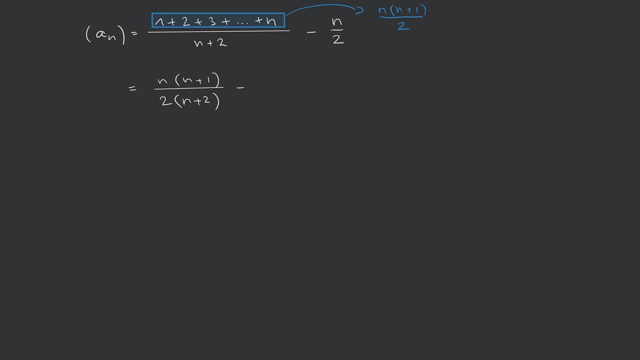 which comes from the blue formula, And we still have minus n over 2.. Now we take things to the common denominator. That means we keep that first expression which has in the denominator 2 times n plus 2.. And the other sum, the minus n over 2, turns into minus n times n plus 2, because we have 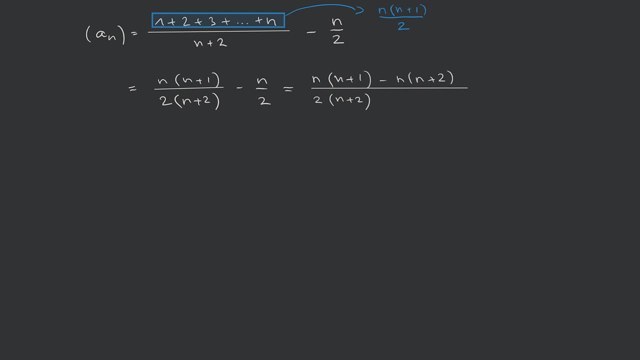 to expand the fraction in order to get the common denominator of 2 n plus 2.. There we go. Now we can simplify the numerator by first expanding the multiplications, which is n squared plus n minus n squared minus 2, n over 2 times n plus 2.. And that simplifies Well, because these two cancel. 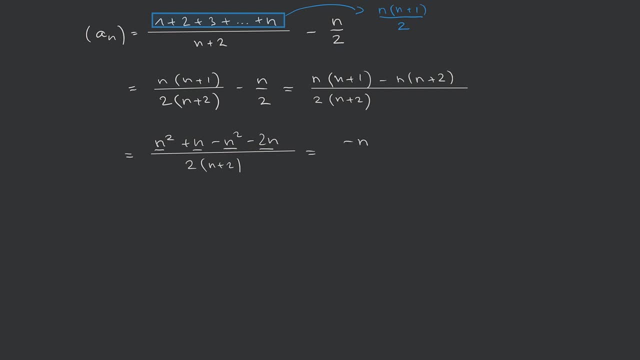 out and these two give minus n. So we have minus n over 2, n plus 4.. So by expanding the multiplication in the denominator Now we apply our standard procedure of identifying the highest power of n and reducing the fraction by this highest power. In this case it is simply n. 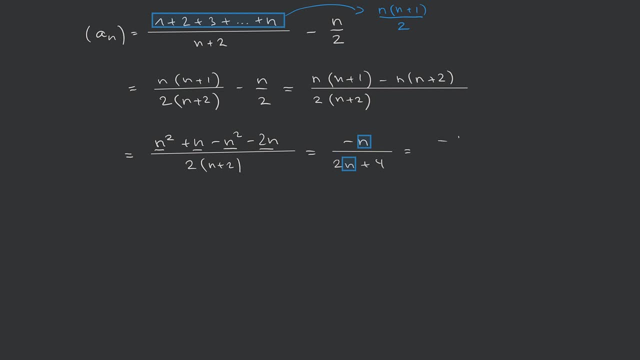 which is why we reduce the fraction by n. So we have minus 1 over 2, plus 4 over n. Now, as always, 4 over n is a zero sequence And we can write that if n goes to infinity, this all goes to. 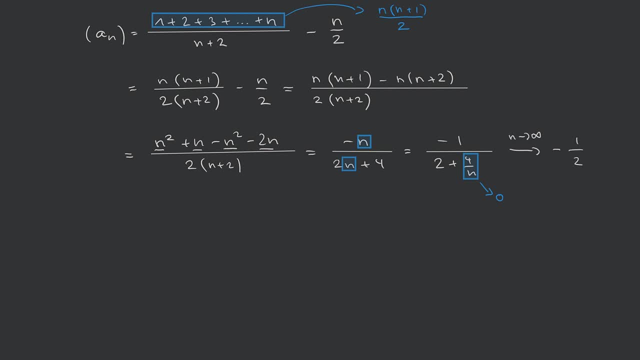 well, what remains? That is minus 1 over 2, so minus 1 half. Now, for those of you who are still not asleep, we're doing another one. a? n equals 2 plus 2 to the second power, plus 2 to the third power. 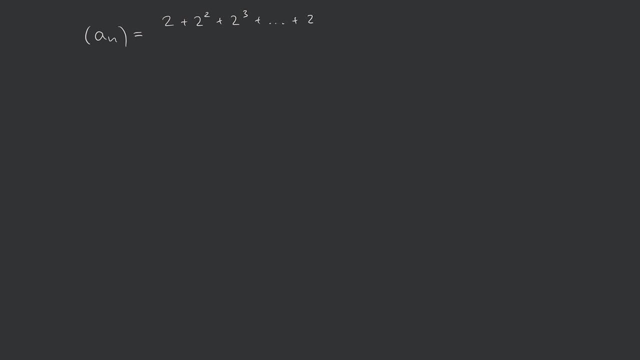 plus dot, dot, dot. plus 2 to the nth power, divided by 2 to the n plus first power, Well, so many powers of 2.. Now the first thing is we train ourselves in using the summation notation. So we replace the numerator by an expression using 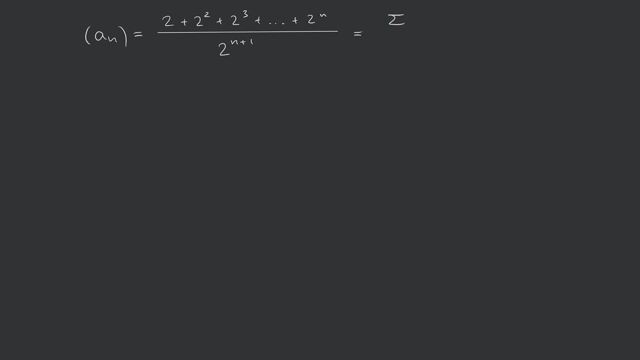 the summation notation. So that is some symbol 2 to the power of i, And now we carefully have to check from where to where i is running. The first summand is 2, which is 2 to the first power. 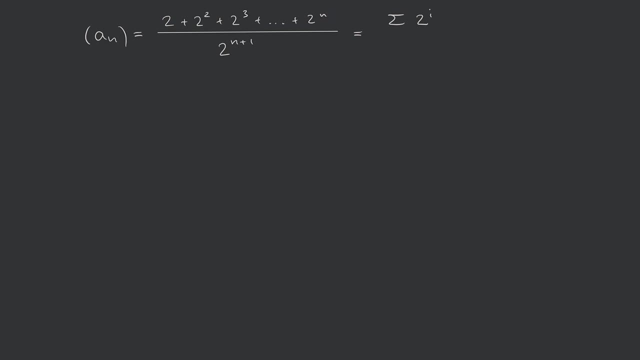 And the last summand is n, So i is running from 1 up to n. And we divide this by 2 to the n plus first power, And we divide this by 2 to the n plus first power, And we divide this by 2 to the n plus first power. 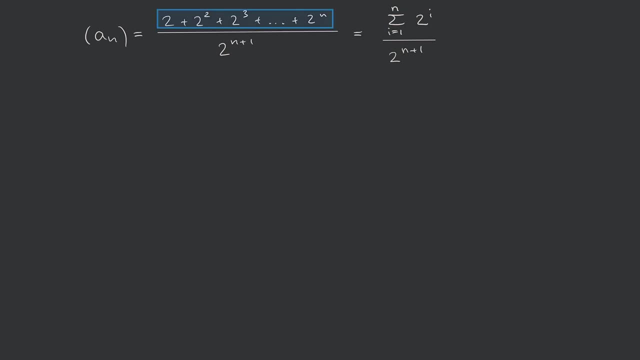 Now something should feel familiar about the expression in the blue box, At least if you've recently watched my video about geometric series. In that video about geometric series, we have shown that whenever we have a geometric series which is given by some q to the power of i- where i runs- 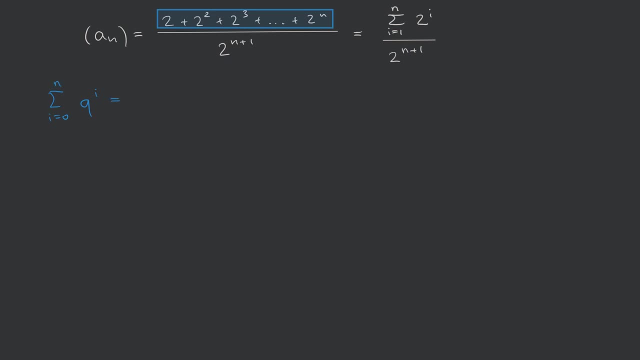 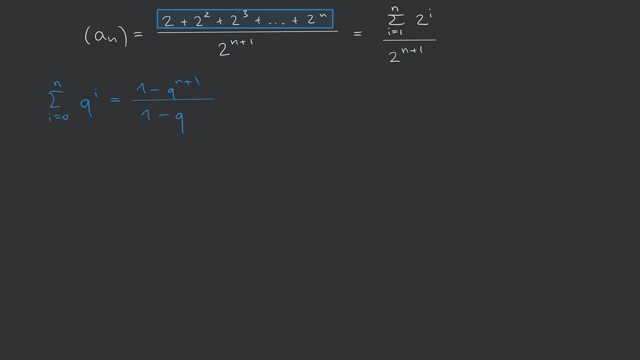 which is 1 minus q to the power of i, which is 1 minus q to the power of n, plus 1 over 1 minus q. So that is C video on geometric series. But that means we can apply that formula to the numerator. 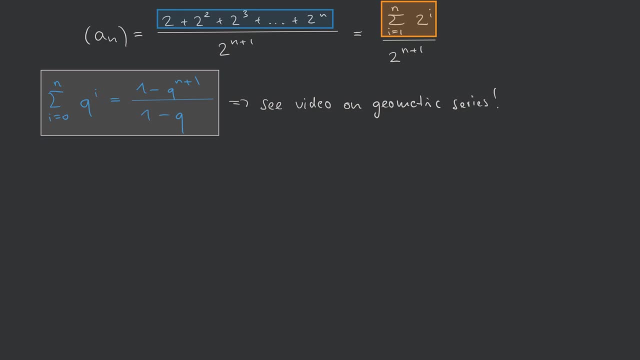 But if we watch very closely, we see that there is a slight difference between the expression in the orange box and the formula for the geometric series. The difference is that the summation index in the expression of the orange box starts at 1.. Whereas the summation index in the formula for the geometric series starts at 0.. 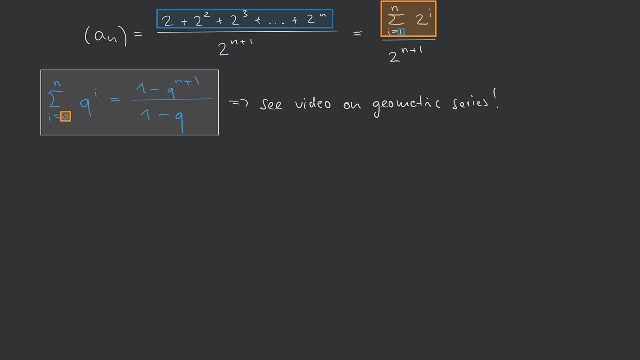 So we cannot directly apply the formula for the geometric series to the orange box. However, we could modify the expression in the orange box such that the summation index starts at 0. And of course we have to redo that modification afterwards. So in fact, what do? 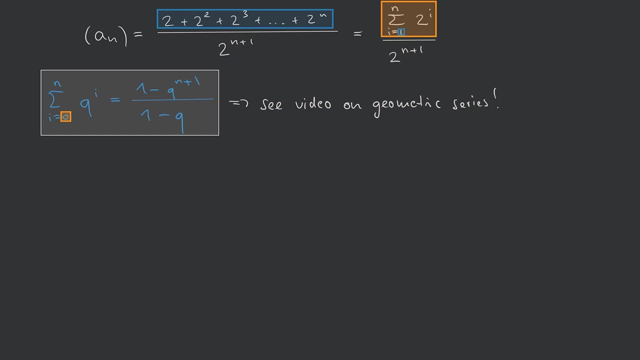 we need to do? to start at 0?? Well, we have to add the number 1 to that sum, which is nothing else than 2.. To the power of 0. That is the missing thing. So we do the following: This equals sum over. 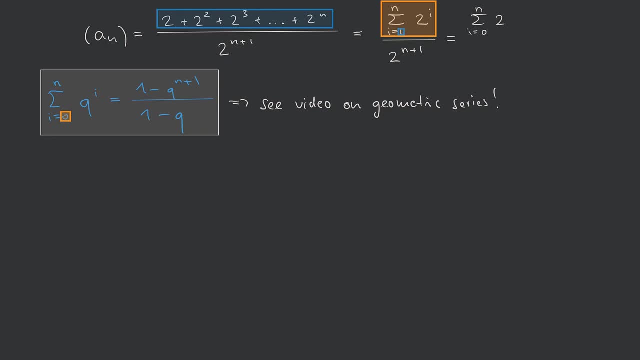 now i, starting at 0 to n, 2 to the power of i, And now we have to redo the thing we've changed, and that is we have to subtract the number 1 again. Now we divide this by 2 to the power of. 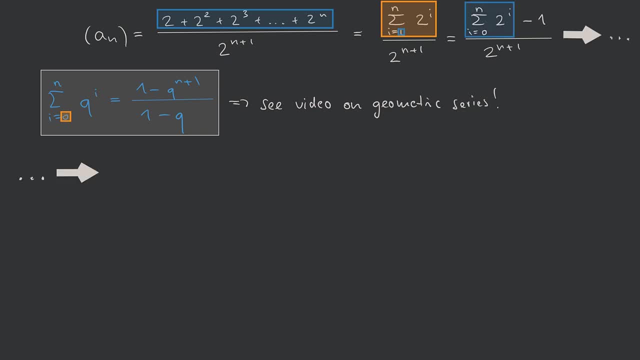 n plus 1.. And we continue down there. So we replace the expression in the blue box using the form, the formula of the geometric series And get 1 minus 2 to the power of n plus 1 divided by 1 minus 2.. 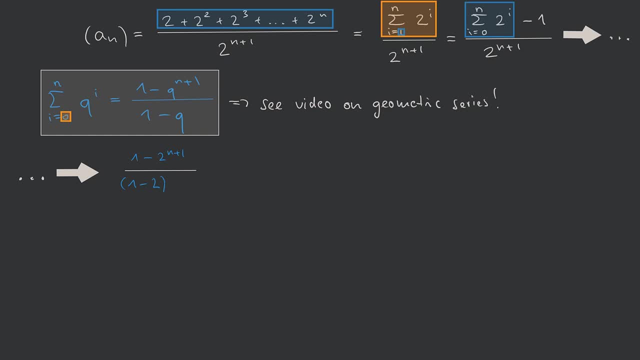 And now we have to multiply that with the actual denominator, which is 2 to the power of n plus 1.. And we have to subtract 1 over 2 to the power of n plus 1.. So you see, I have split up this fraction. 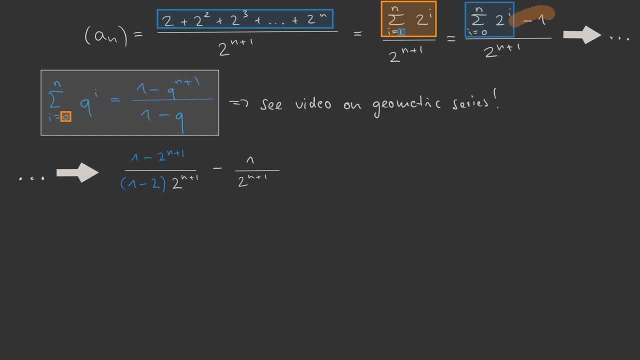 into this part And this part, And in that first part I have replaced the expression in the blue box using the formula for the geometric series. Now the next step. we can simplify things a little: 1 over 1 minus 2 to the power of n plus 1.. Now divide it by so: 1 minus 2 is minus 1.. So we can. 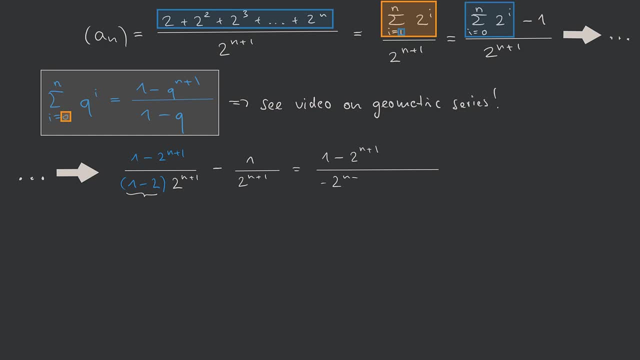 write. so we can write minus 2 to the power of n plus 1.. And now we have this expression: minus 1 over 2 to the power of n plus 1.. And now we have this expression minus 1 over 2 to the power of n plus 1.. 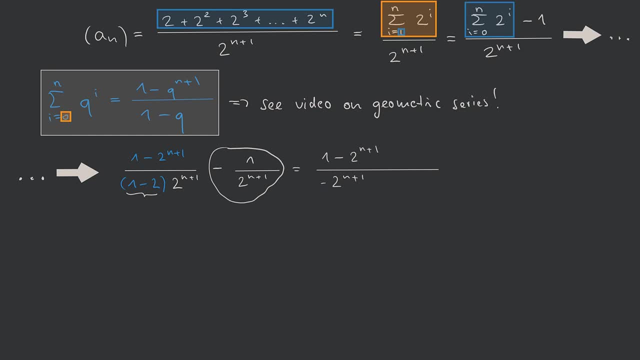 So, except for the minus sign that has the same denominator. So we can change that minus sign to a plus sign like this, And we have taken everything to the common denominator. So we can further simplify: 1 plus 1 is 2 minus 2 to the power of n plus 1, over minus 2 to the power of n plus 1.. 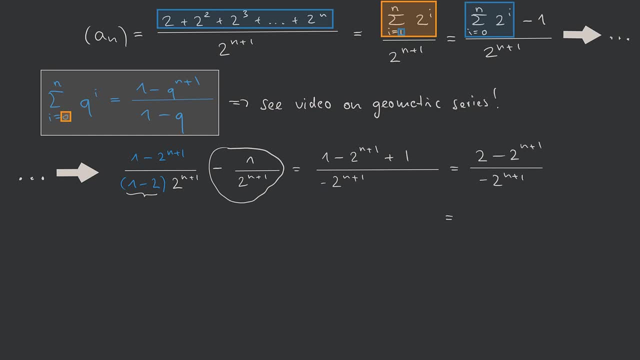 So now we reduce by, let's say by minus 2.. We reduce the fraction by minus 2.. So we have minus 1, now plus, And now 1, now 1 power less than n plus 1, which is n. So only to the power of n. 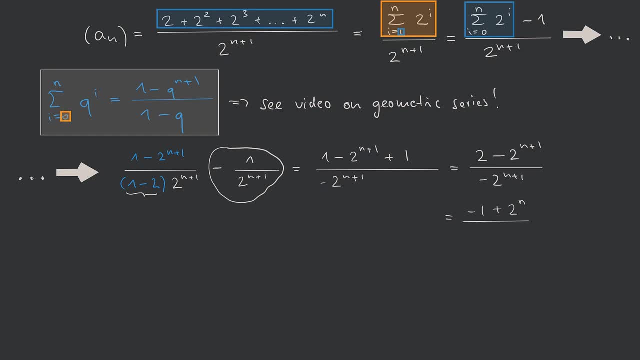 Because we have divided 2 to the power of n by 2. It remains 2 to the power of n And the same in the denominator We reduce by minus 2.. So we have plus 2 to the power of n. Again, we want to create: 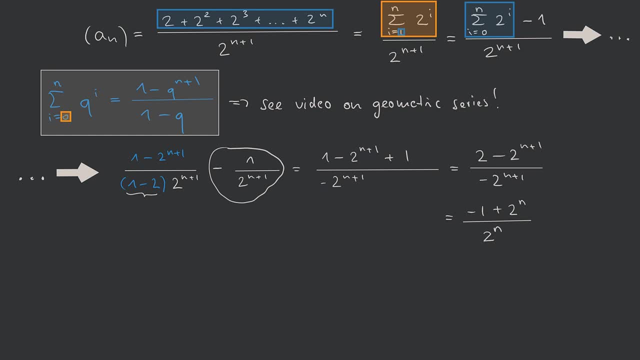 zero sequences. So again we identify- let's say it's not the highest power of n in this case, But generally speaking, the summons which grow fastest. So these summons are two to the power of n, which we have twice. 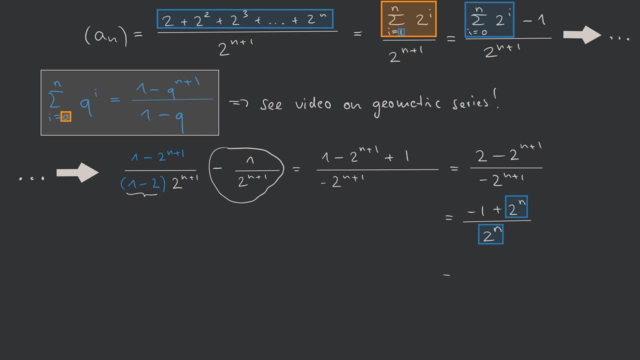 So we take those and we reduce the fraction by those, And I swap the summons in the numerator So we get one minus one over two to the power of n, divided by well, divided by one, And finally we are ready for the showdown. 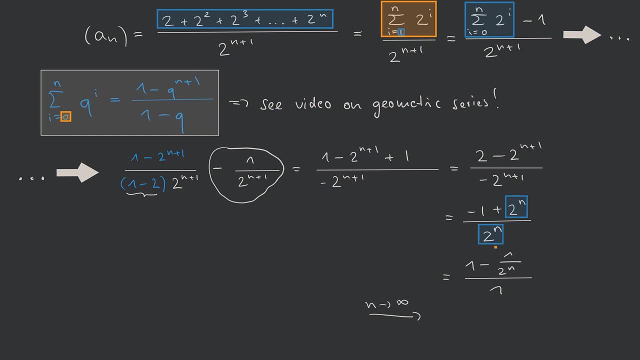 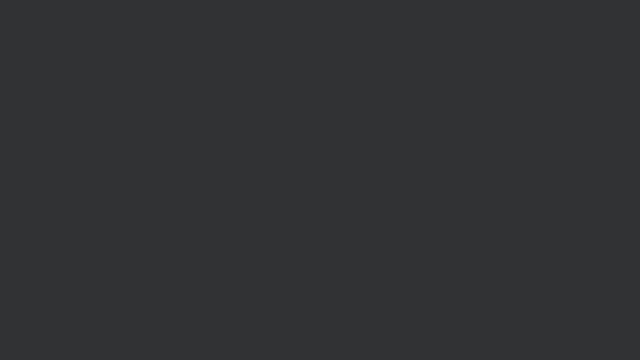 because now, if n goes to infinity, we have that this sequence is a zero sequence, So it goes to zero, which gives us, finally, the limit one for this rather complex sequence. Now, for those of you who made it until this point, I have some very bad news for you. 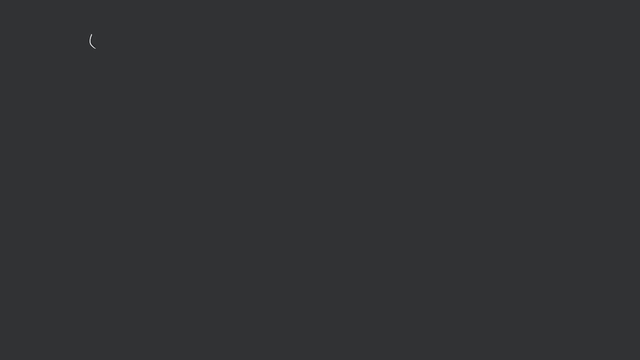 because I have only one example left, And this is the following: an equals one plus 1, 3rd plus one over nine, plus dot dot dot plus 1 over 3 to the power of n divided by something which is very similar, but only 5 instead of 3,. 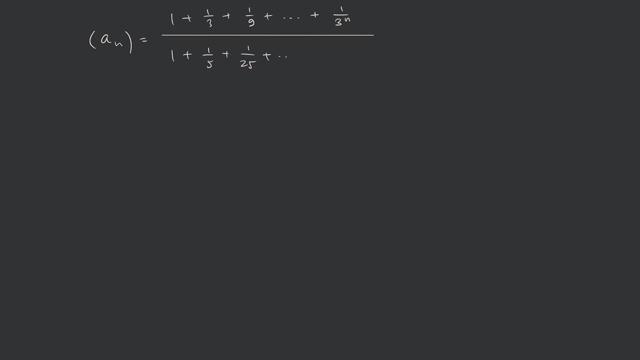 so 1 over 5 plus 1 over 25, plus dot, dot, dot plus 1 over 5 to the power of n. What is the limit of that sequence? Again, as you very carefully paid attention in my video on geometric series, 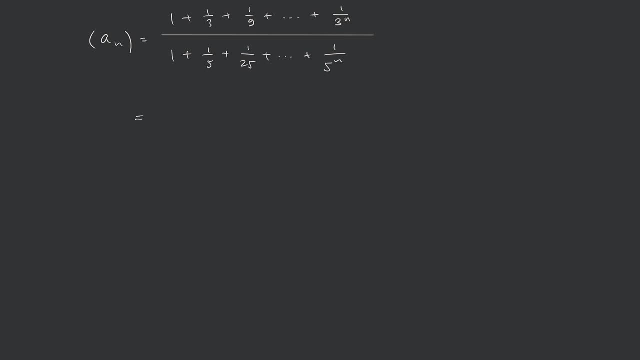 you know that both the numerator and the denominator are geometric series. A geometric series has the general form: i equals 0 to n of q to the power of. i equals 1 minus q to the power of n plus 1 over 1 minus q. And for the special case that the absolute value of q is strictly 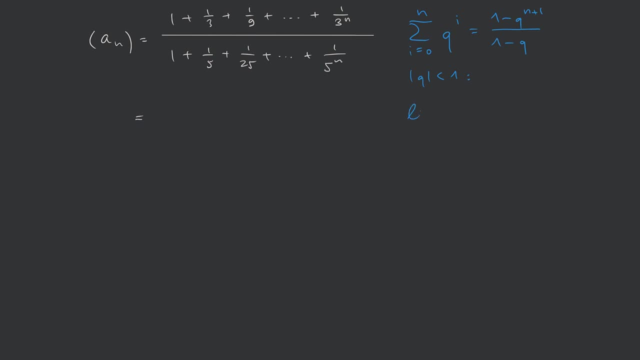 smaller than 1, we have some nice formula for the limit of that sequence, So we can write: lim n to infinity, i equals 0 to n, q to the power of i. Well, that was 1 over 5.. 1 over 1 minus q. So that is the story about geometric series And we can apply that here. 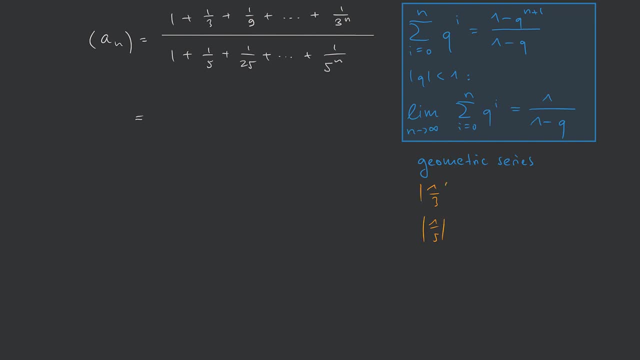 because one third and one fifth are both numbers whose absolute values are strictly smaller than 1.. So we can calculate the limits for both the numerator and the denominator by using this formula. So I can write: lim a n- for n goes to infinity- is equal to lim of. 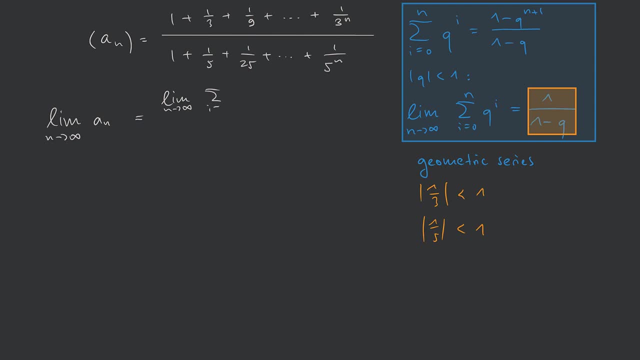 n. Well, let's write it like this: n to infinity i equals 0 to n, one third to the power of i. just using summation notation to in fact make things easier in this moment, and divided by structurally the same thing, lim n to infinity, sum over i equals 0 to n. now, one third replaced. 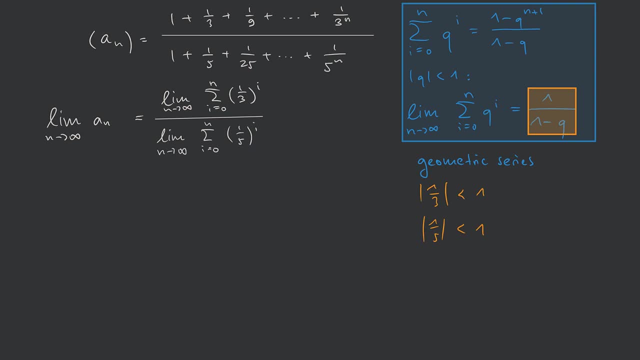 by one fifth to the power of i. Now, in both cases the numerator and the denominator- we can use that orange box over here in order to write that in a much simpler way, because that is well 1 over, 1 minus q, but q in this case is one third, So 1 minus one third. 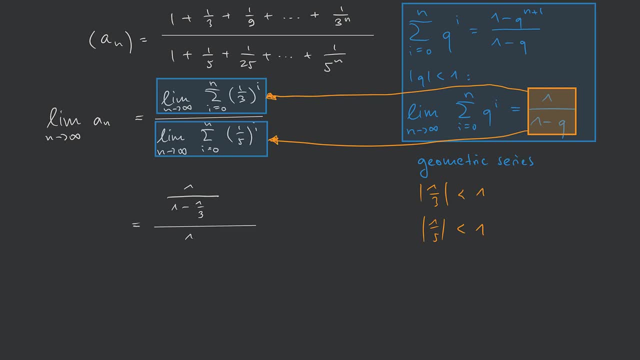 Now that looks like a double whopper divided by, and the same thing is in the denominator, So 1 over 1 minus one fifth in this case. Now we have to resolve that double whopper, which is not hard because 1 minus one third. 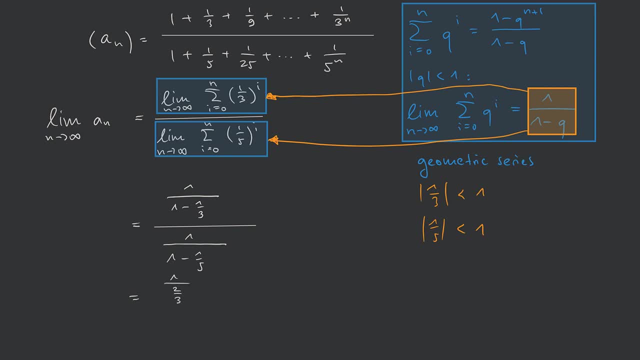 is two thirds, So we have 1 over two thirds over 1 over four. fifth, That is funny, isn't it? And that equals well, 3 over 2 over 5 over 4, and that equals 3 over 2 times 4 over 5.. Now we 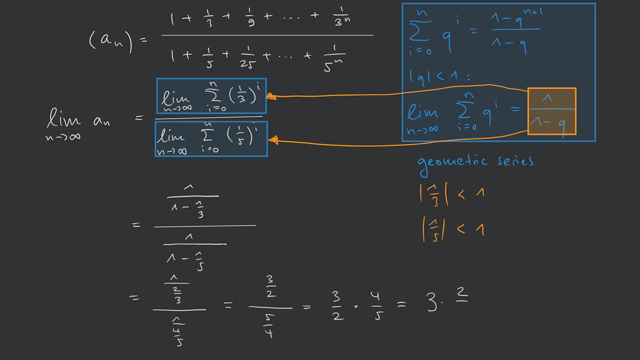 can reduce by 2,, which is 3 times 2 over 5, and that is 6 over 5.. There we go. That is the limit of that funny sequence. So well, those of you who made it until here, I am very happy that you followed me on that. 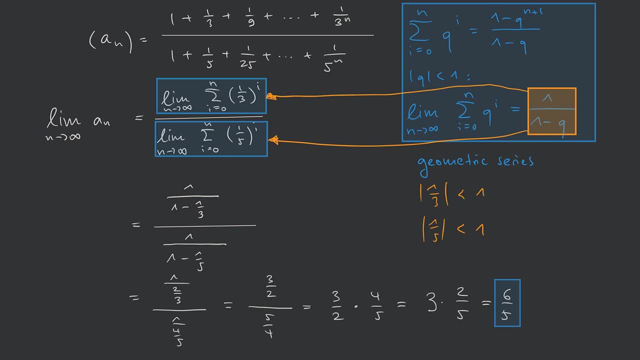 journey. Actually producing that video took me two days, So that's the end of two days work, and I'm really relieved that I did it. So all remains is to say thanks a lot for watching that and see you next time. Bye-bye.